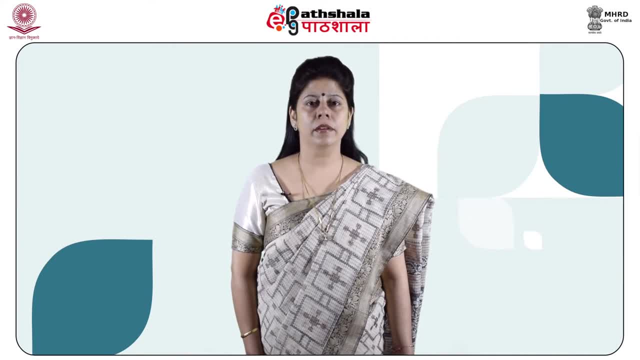 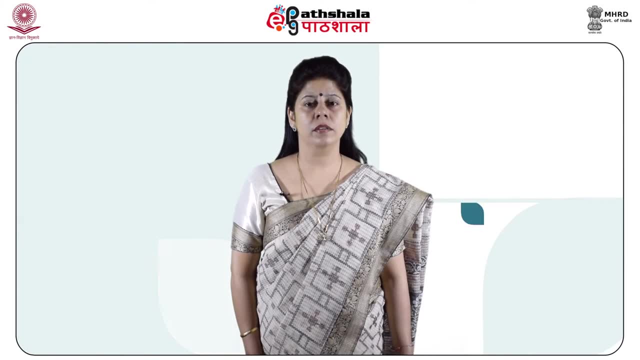 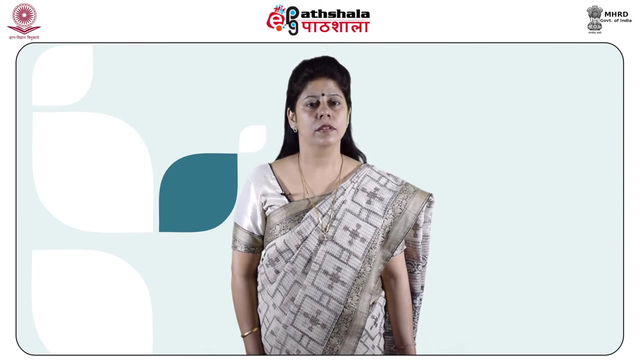 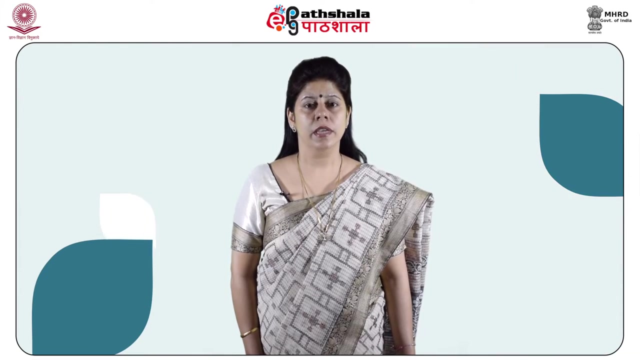 and their effect on the environment and the mankind. Let us see the pollution from heavy metals. The problems of pollution from heavy metals affects the whole population and considers all the three receiving section. The principal emission sources come from the industries such as petrochemicals, extractive. 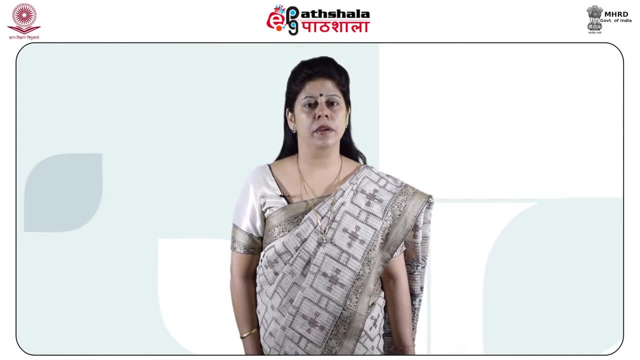 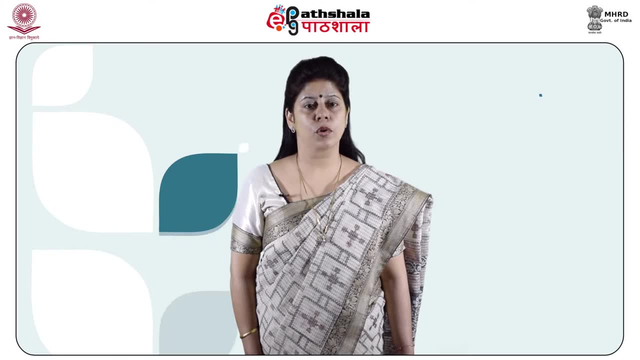 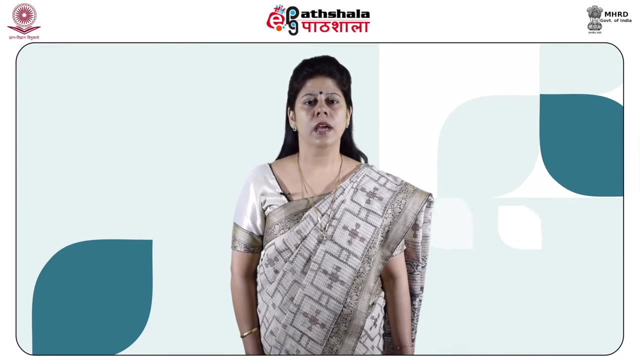 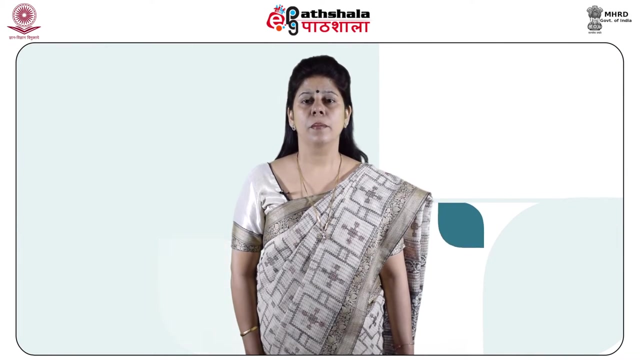 metallurgy, mechanic, chemicals and ceramic. However, the current module mainly emphasizes on the heavy metal, soil pollution and its adverse effects. Metal as soil pollutants. Metals are the natural substances that are formed in the soil at low levels. Nevertheless, the metals emitted by the processes such as mining, manufacturing and the use 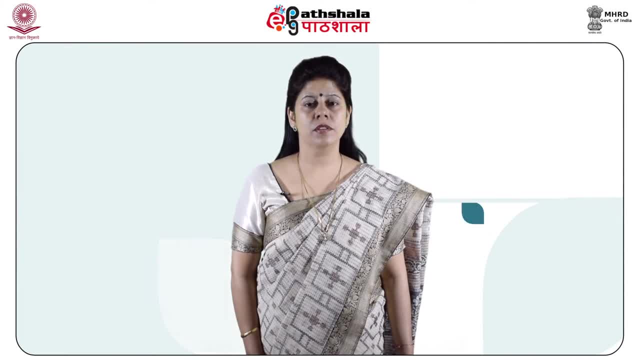 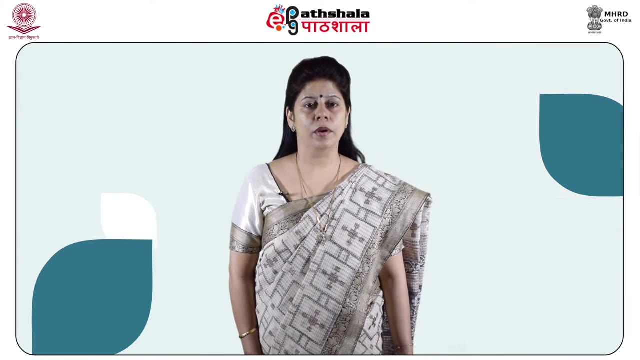 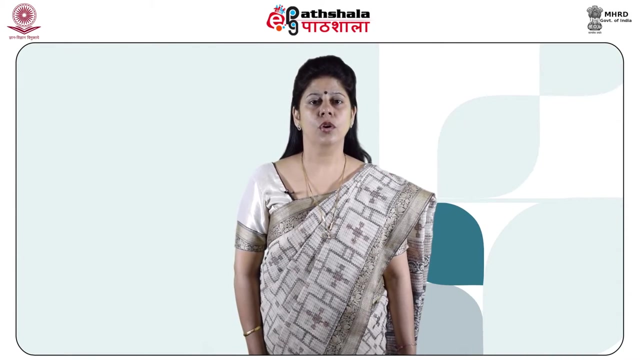 of synthetic products result in contamination in urban and agricultural soils. They remain in the soil indefinitely, As the metals don't degrade. Excess concentration of heavy metals in soil, by direct or indirect means, can transfer through food chain and are toxic for human health and environment. The problems associated with continuous exposure to heavy metal results in mental lapse due to lead. Cadmium affects kidney, liver and gastrointestinal system. Acidic smile, masturbation and gastrointestinal tract. arsenic leads to the skin poisoning effects, kidney and central nervous system and many more diseases are possible due to. 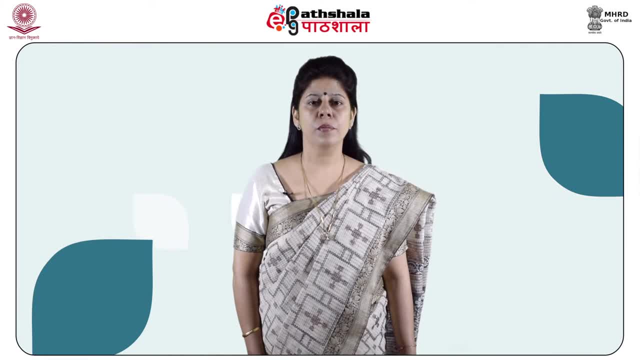 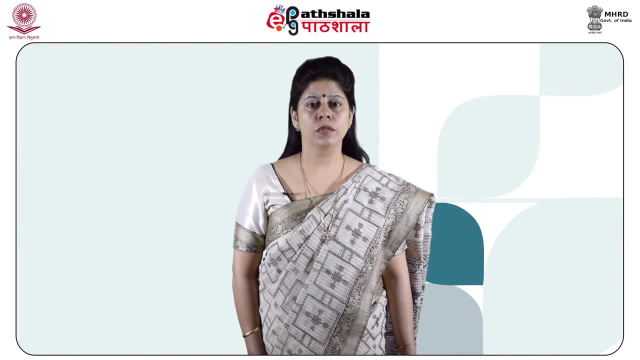 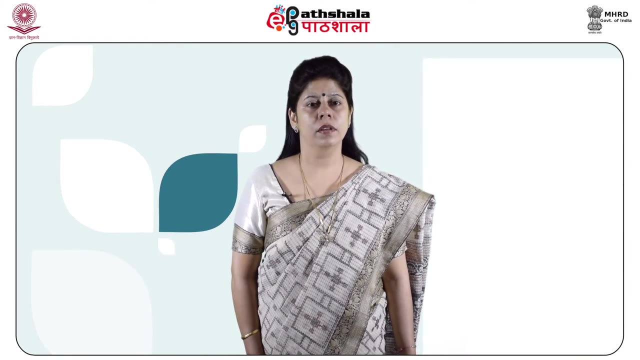 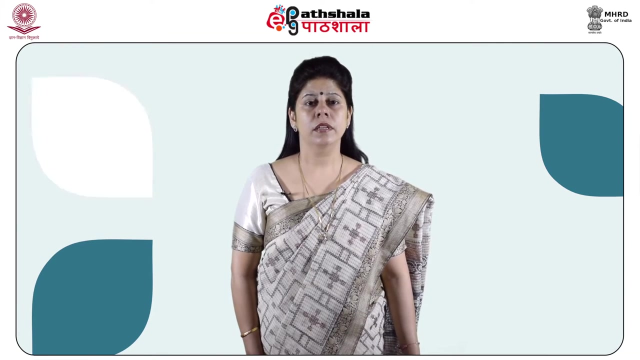 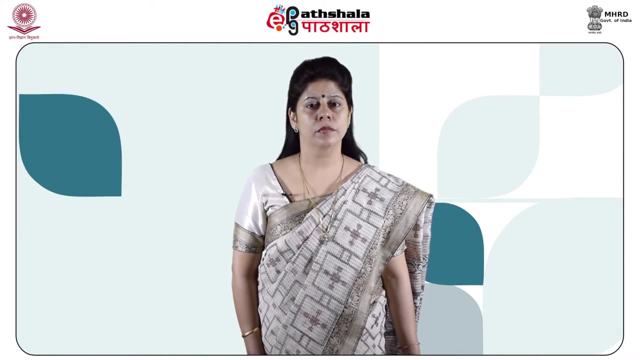 think that today we're spending loves and excess metal. Acute toxicity From exist in soil as positively or negatively charged species. Mercury, cadmium, lead, nickel, copper, zinc, chromium and manganese are cations in the soil. On the other hand, arsenic, molybdenum, 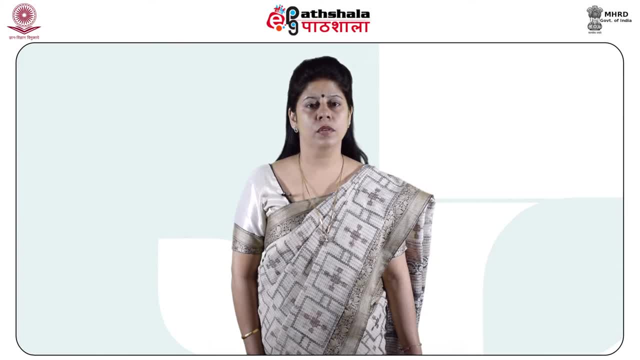 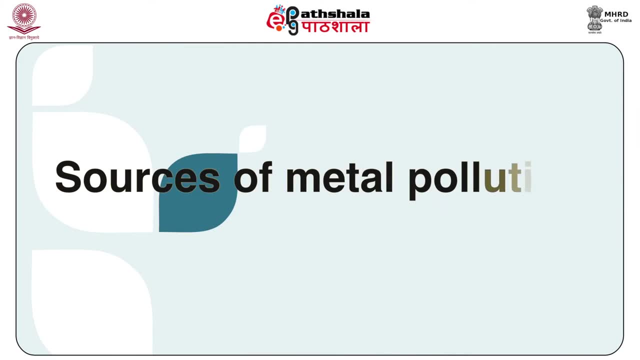 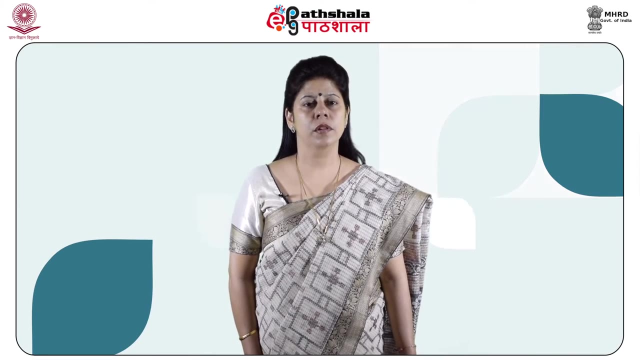 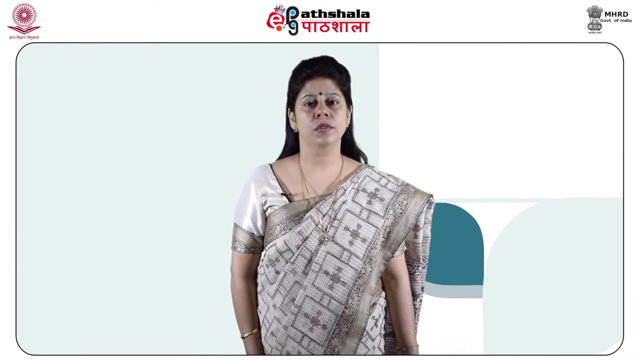 selenium and boron are the anionic compounds in the form of arsenates, molybdates, selenides and borates. Sources of metal pollution: Natural and anthropogenic. both the sources are responsible for environmental pollution which are hazardous to environment. Some of the natural sources. 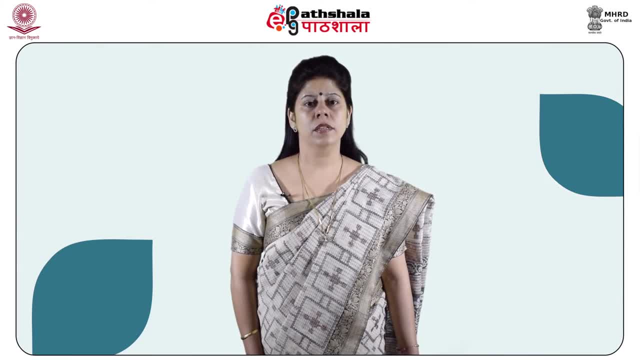 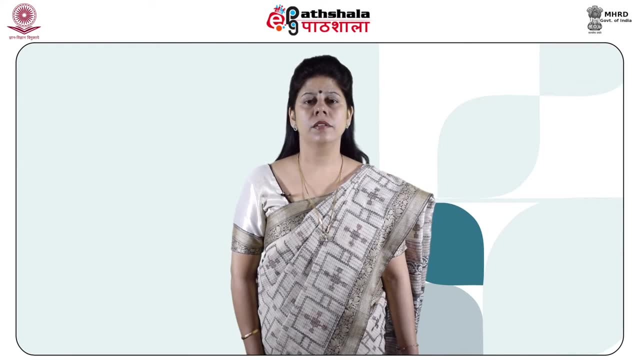 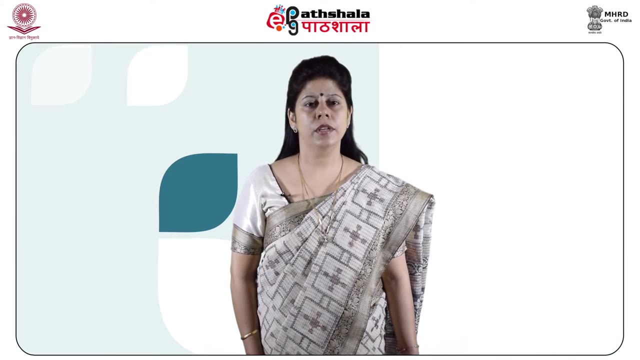 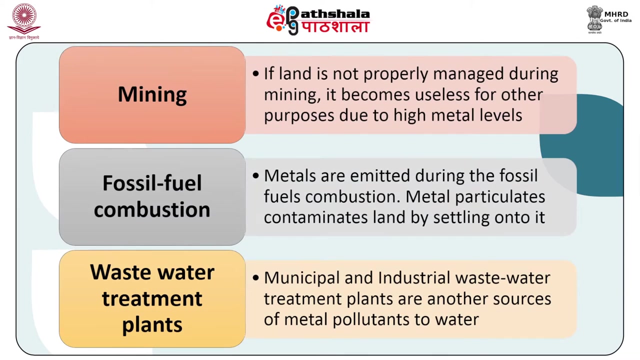 include volcanoes, forest fires, seepage from rocks into water, sea salt sprays, etc. These are significant, but it is human nature to do so, Human activity that are more responsible for an increase in the metals into the environment. Some of such activities include mining, in which, if land is not properly managed during 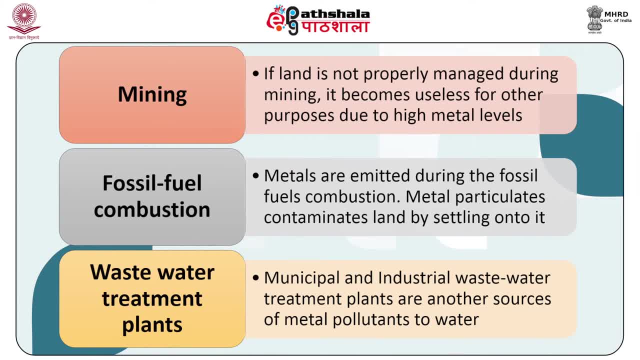 mining. it becomes useless for other purposes due to the high metal levels. Second, the fossil fuel combustion Metals are emitted. during the fossil fuels combustion, metal particulates contaminates the land by settling to it. Next, the Municipal and Industrial waste water treatment plants are the another source. 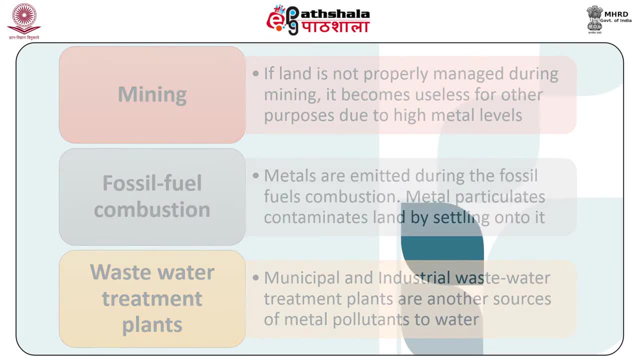 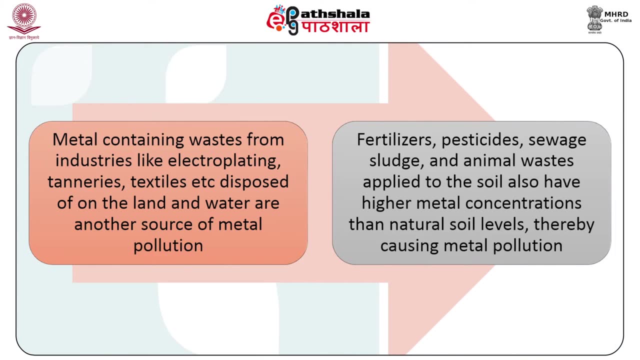 of the metal pollutants to water. Next, metal-containing waste from industries like electro-plating, tanneress, textiles, etc. being disposed on the land and water. Some necessary sources for metal pollution can be found: Aerial photosynthesis, Acetate septic, einen Triglyceride. 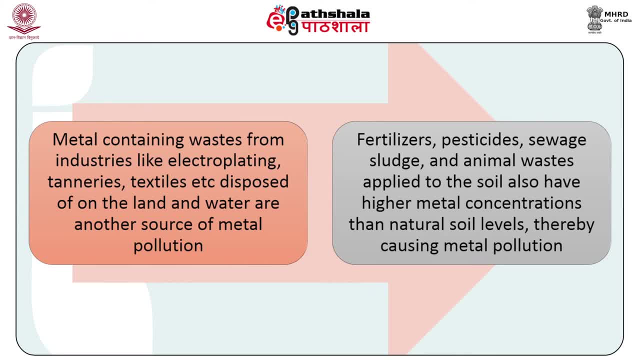 alum Nicholas corona Prypter. What is dioxide? Non-oxidant might be the solution for Site A in plants. Malaria. most package of Aquatic are another source of metal pollution: Fertilizers, pesticides, sewage sludge and animal waste. 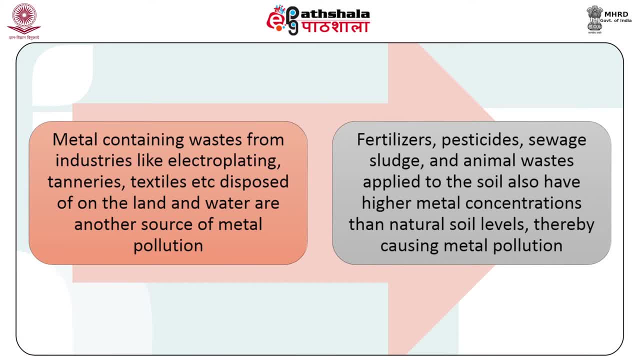 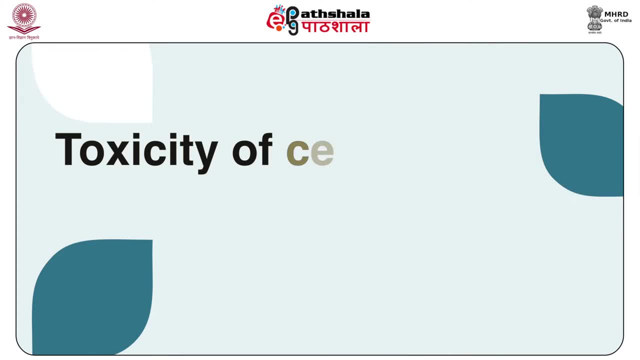 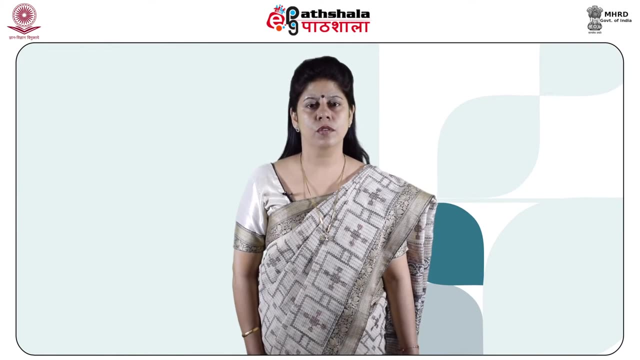 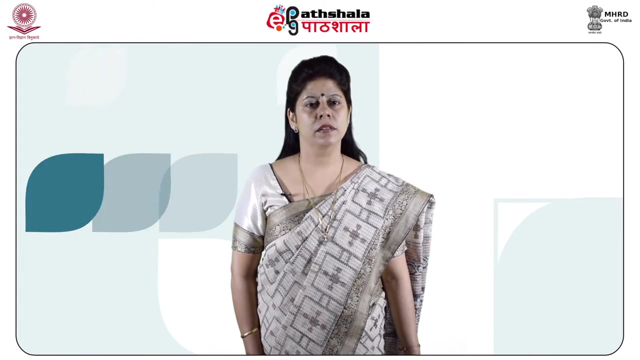 applied to this soil also have higher metal concentration and natural soil levels, thereby causing metal pollution. Now let us see the toxicity of certain metals. Metabolical toxicity is a deadly effect of certain metals in definite forms and doses on life form. Some of the metals are very toxic as they form soluble compounds, poisonous. 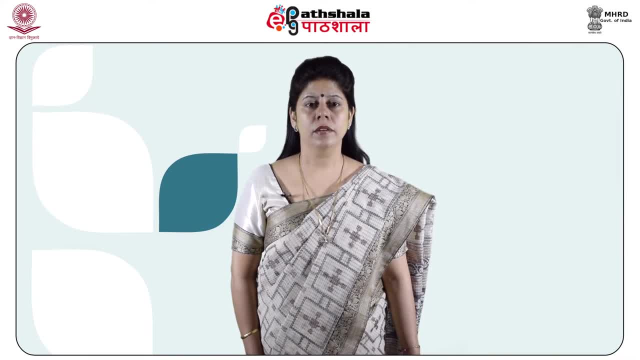 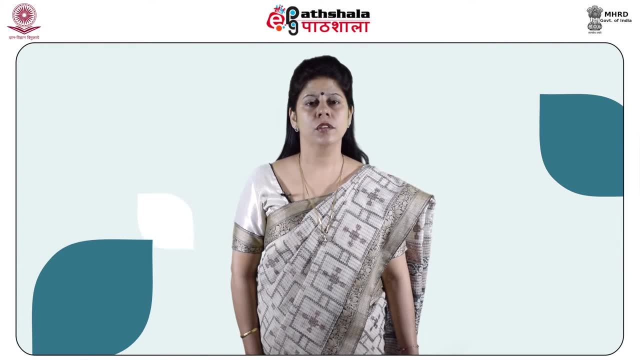 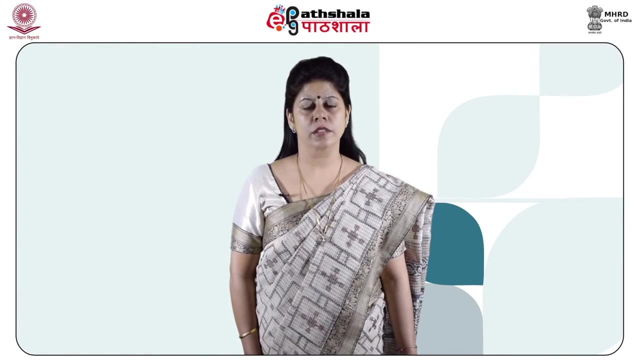 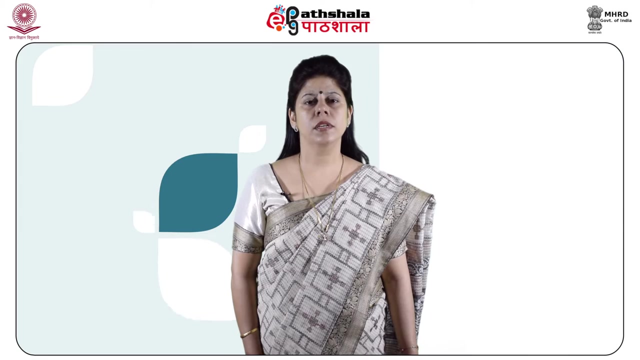 in nature. Some toxic metals replicate the action of essential elements in the body, thereby interfere with the metabolic processes to cause illness. It includes cadmium, lead, mercury and radioactive metal. Now let us see the toxicity caused by lead. The Minnesota State Legislature has recognized 100 ppm of lead as a bare soil standard. The Environmental Protection Agency of United States and most other states uses more than 100 ppm level of lead. Around 300 ppm level is used, based on the level of lead used in food chain poisoning. This is based on risk measures on eating of soil by young children. 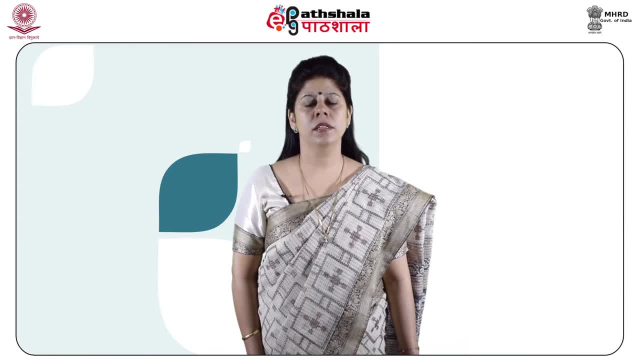 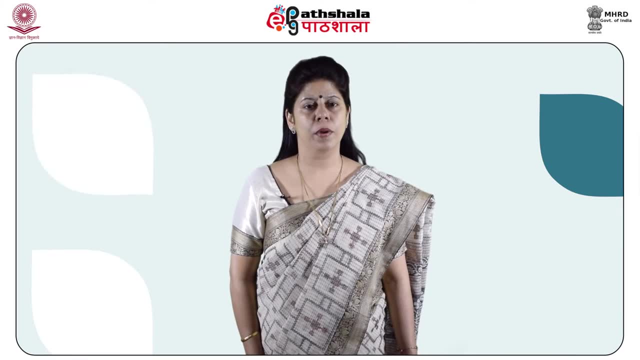 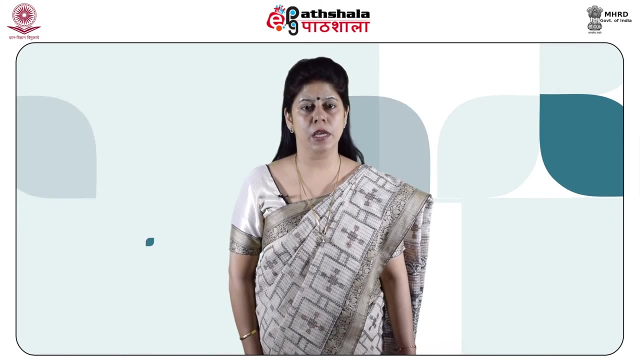 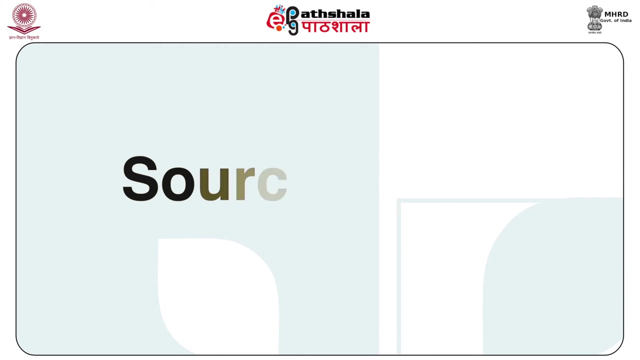 Since the soil, lead is not taken by plants in large quantities. therefore, the level of lead in soil is not dangerous for plants. Generally, the soil having total lead levels less than 300 ppm is safe, but as the level increases it results in lead poisoning via food chain. 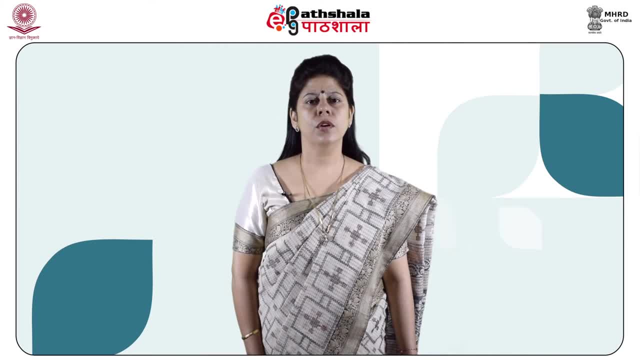 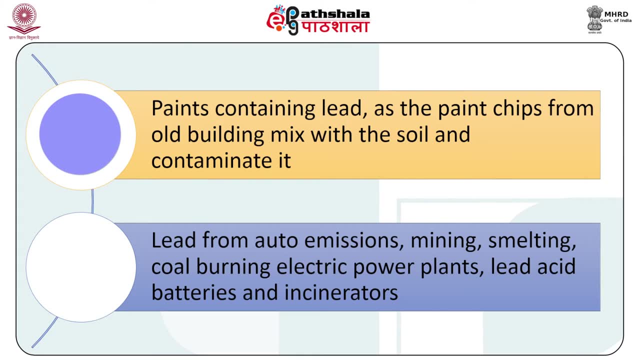 Now we will see what are the sources of lead. The sources of lead contamination are: paint containing lead, as the paint chips from old building mix with the soil and contaminate it. The lead from auto emissions, mining, smelting, coal burning, electric power plants. 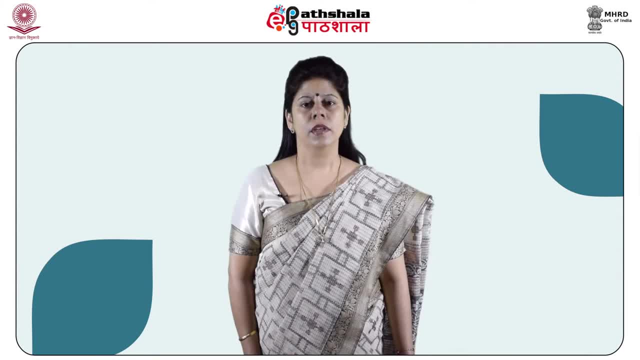 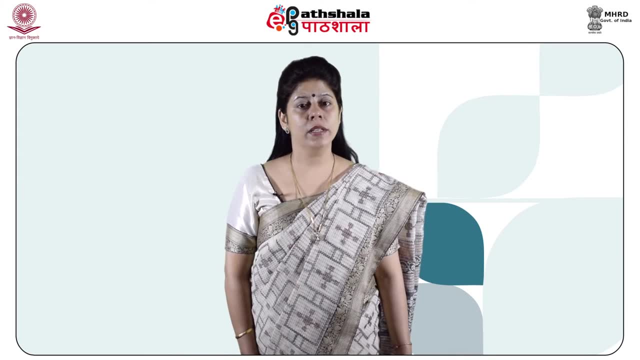 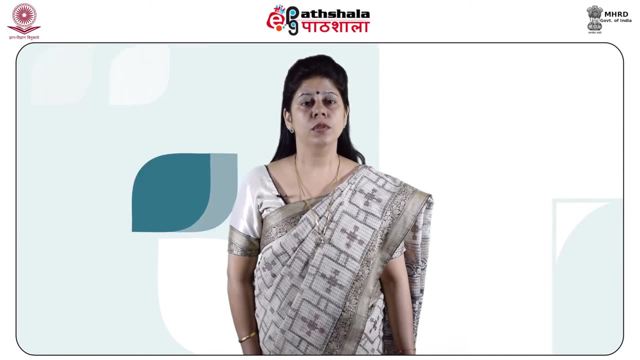 lead acid batteries and incinerators. In present time, the level of lead in paints and gasoline is quite low, but once it gets deposited on soil it can persist for a long time. Therefore, to some extent, these are the source of lead contamination. Generally, the lead is not absorbed. 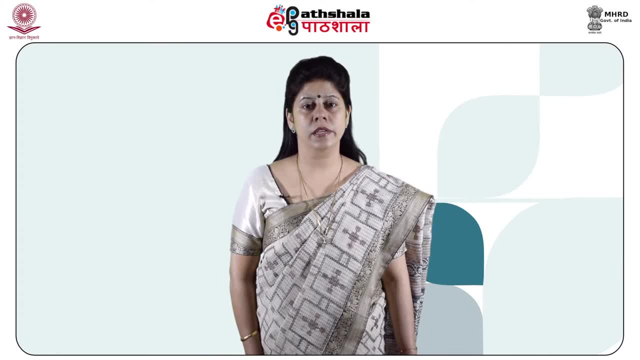 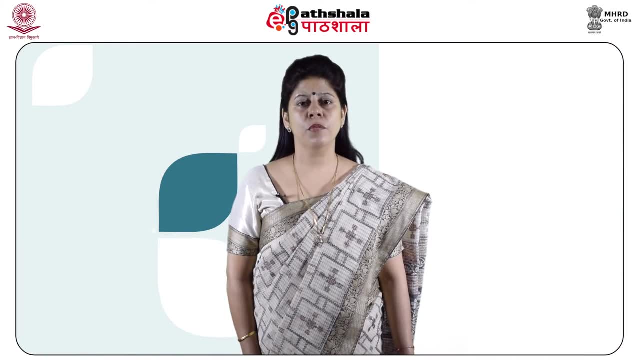 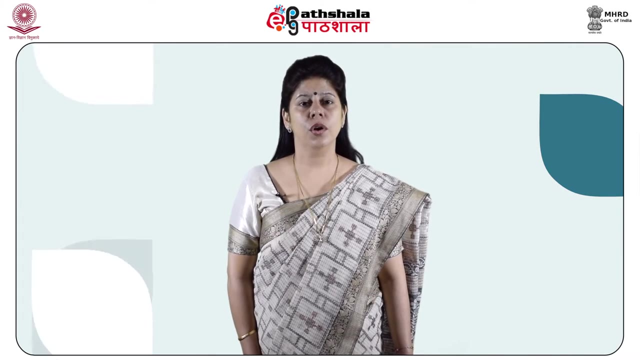 by plants, But if soil contains high lead content, plants can take up some amount of it. It is estimated that sometimes lead can be absorbed by plants in different ways, For some crops like corn beans, squash, tomatoes, strawberries and apples are not readily contaminated. 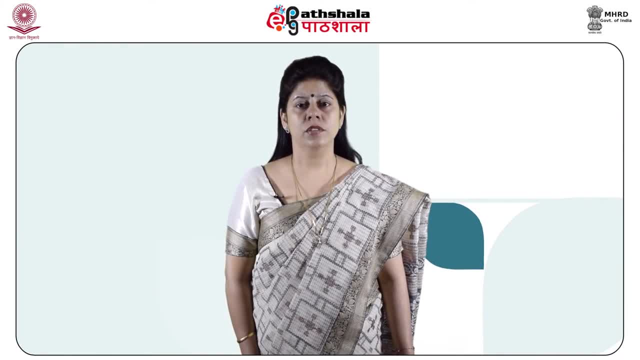 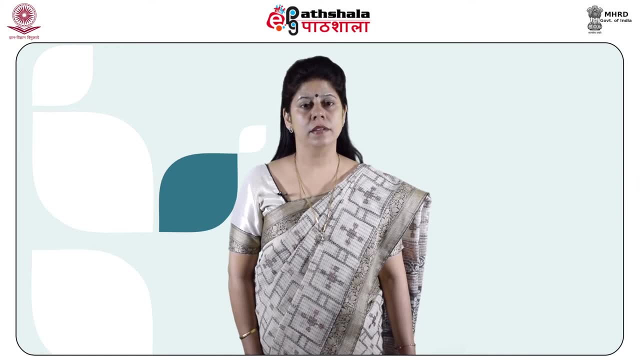 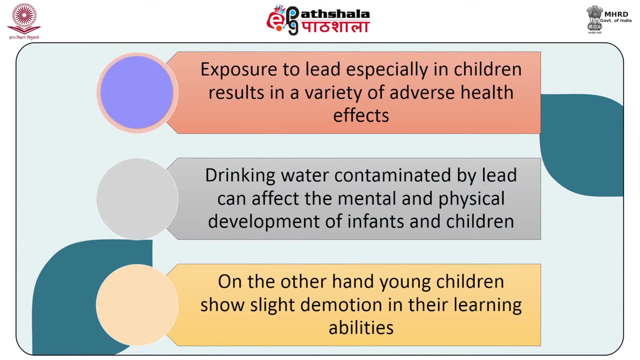 by lead, But leafy vegetables such as lettuce and root crops like carrots are likely to be contaminated by the lead in high concentration. Now we will see what are the health effects caused by lead exposure. Exposure of lead, especially in children, results in a variety 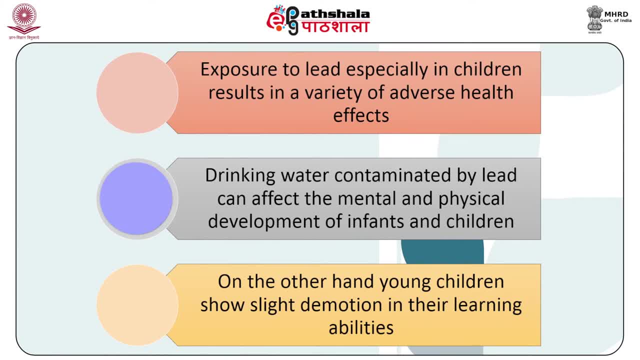 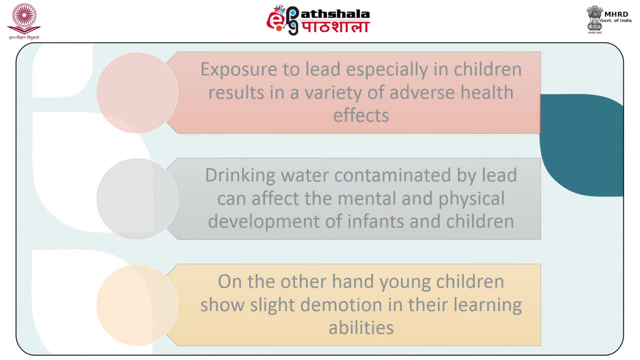 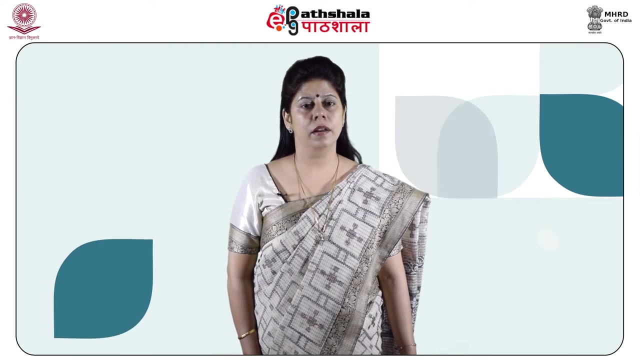 of adverse health effects. Drinking water contaminated by lead can affect the mental and physical development of infants and children. On the other hand, young children show slight demotion in their learning abilities. In adults, the continuous exposure of lead may result in kidney and high blood pressure problems. They can also have fertility problems and 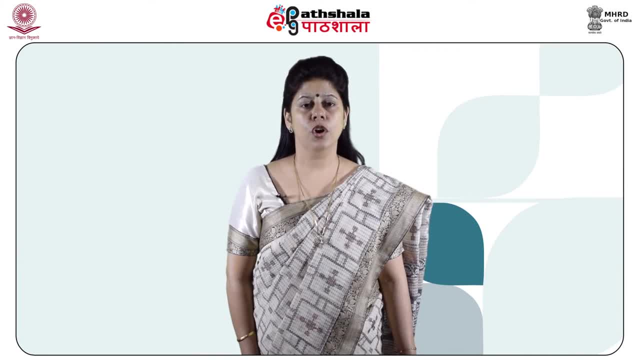 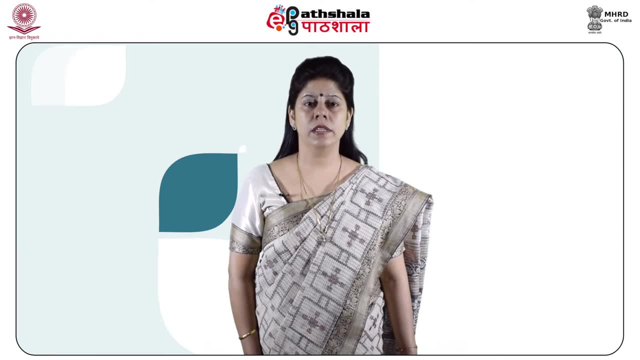 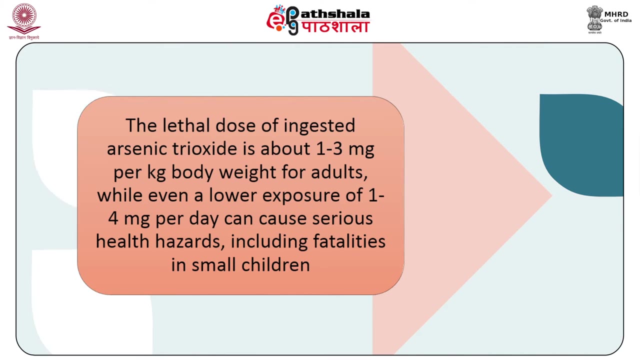 cataracts. Other symptoms are abdominal pain, anemia and lesions of central and peripheral nervous system. Now we will see another metal, that is arsenic. The lethal dose of ingested arsenic trioxide is about 1 to 3 mg per kg body weight for adults, while the lethal dose 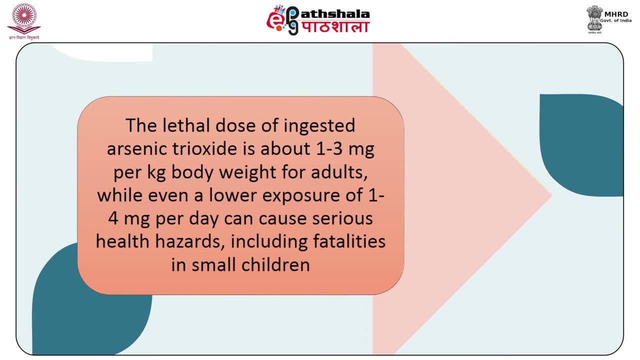 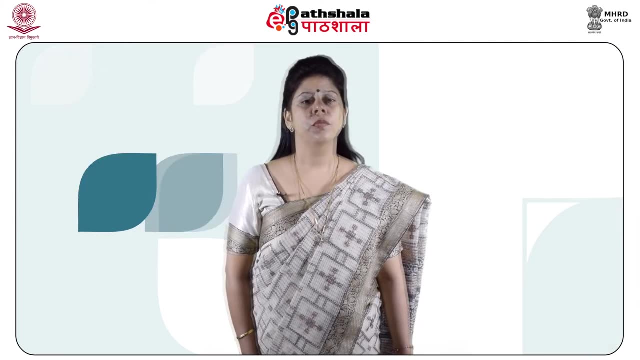 of arsenic trioxide is about 1 to 3 mg per kg body weight for children, While even a lower exposure of 1 to 4 mg per day can cause serious health hazards, including fatalities in small children. The concentration of arsenic is highest in the contaminated water From many. years. coal-based power plants, ore smelting operations and inorganic arsenic chemicals that are used in agriculture results in contamination of soil. In addition, the use of arsenic in local areas by introducing arsenic oxides, The inorganic arsenical pesticides and oxides. 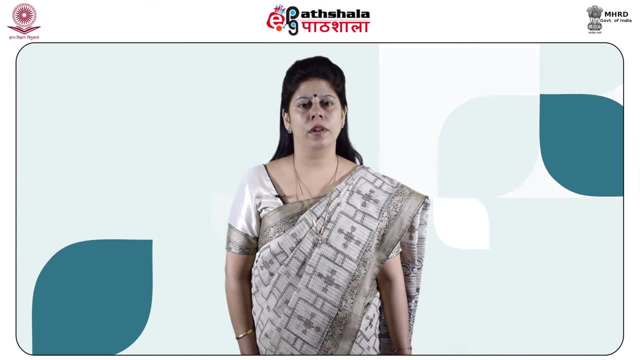 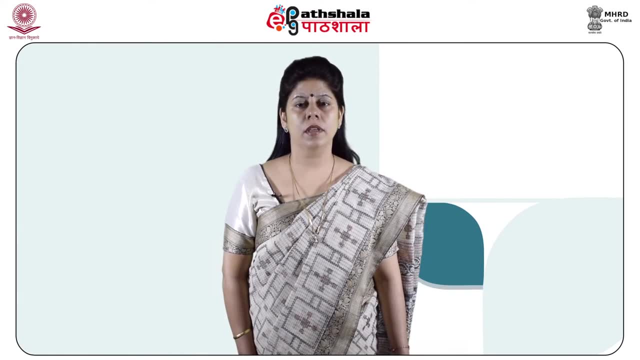 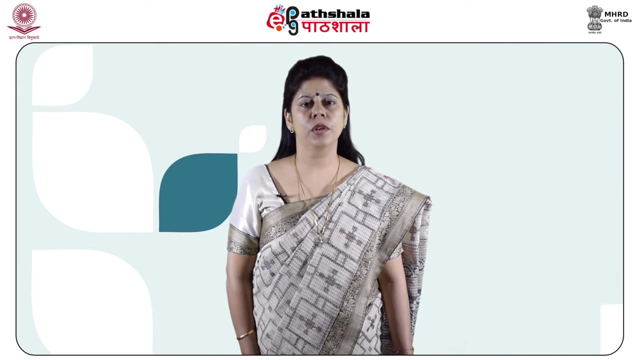 of arsenic, when incorporated into the soil under oxidation conditions, get converted into arsenates. In some properties, the arsenate ions is similar to ortho-phosphate and can be absorbed by iron and aluminum components. This will affect the deposition of arsenic in the soil. In some properties, the arsenic ions are similar to ortho-phosphate and can be absorbed by iron and aluminum components. This will affect the deposition. 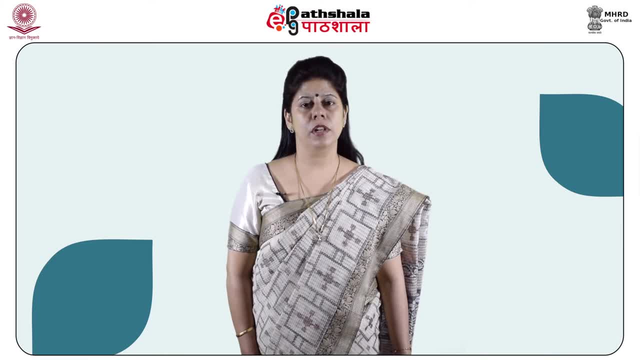 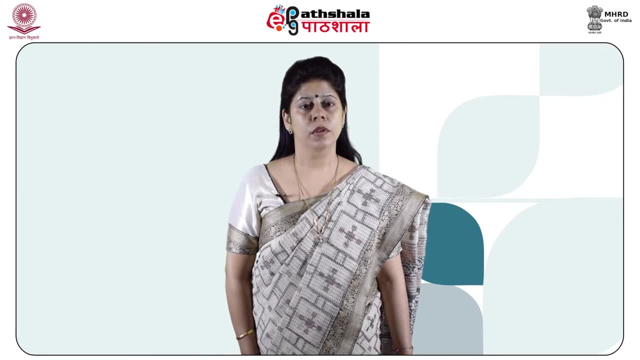 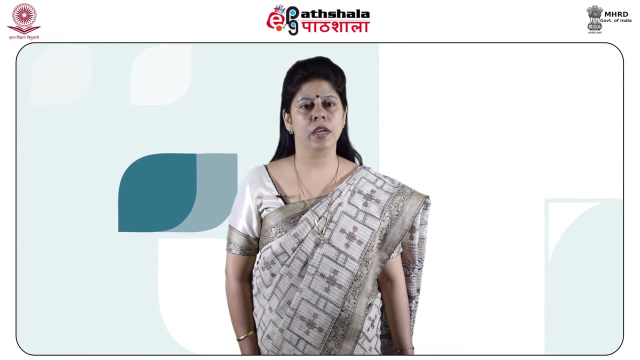 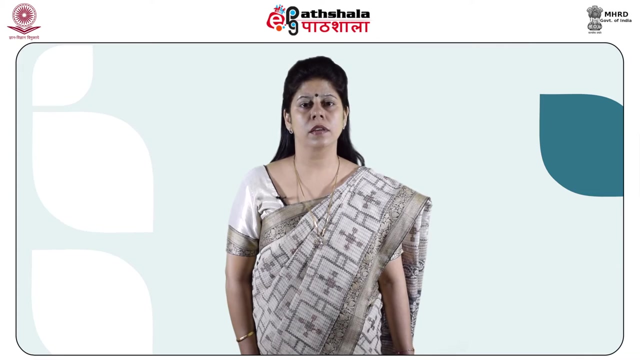 of arsenic in the soil and hence its availability to the plants. Smelting industries contribute in arsenic exposure. Also, the micro-electronic industries, coal power plants, use of pesticides and glass manufacturing treat arsenic as a preservative. Now we will see what are the health effects caused by arsenic exposure. Arsenic, is said. 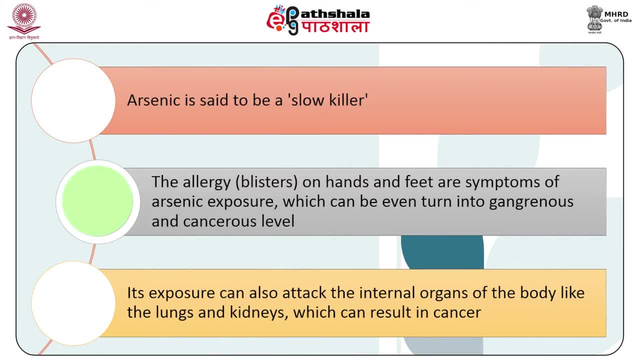 to be a slow killer. The allergy, the acidity, the acidity of the acid, the acidity of the acid. the allergy on the hands and feet are symptoms of arsenic exposure which can even turn into gangrenous and cancerous level. Its exposure can also attack the internal. 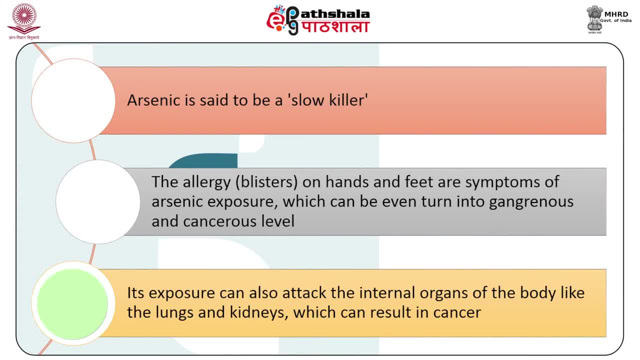 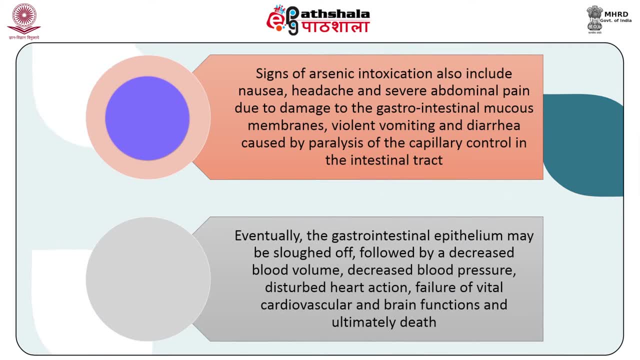 organs of the body like the lungs and kidneys, which can result in cancer. Signs of arsenic intoxication also include nausea, headache and severe abdominal pain due to damage to the body. In some properties, the arsenic ions are similar to ortho-phosphate and arsenic. 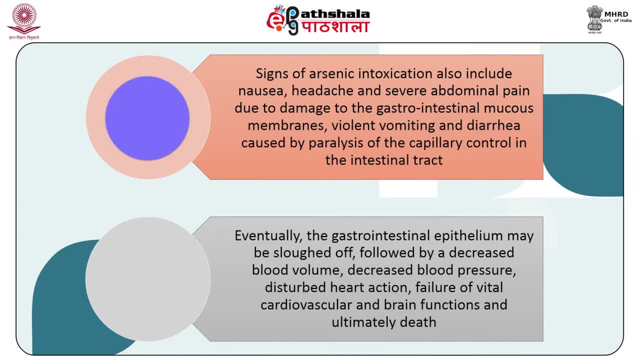 ions are also found in the gastrointestinal mucous membranes. 3.Voilant vomiting and diarrhea caused by paralysis of capillary control in the intestinal tract. Eventually, the gastrointestinal epithelium may be slugged off, followed by a decreased blood volume, decreased blood pressure, disturbed heart function, failure of vital cardiovascular. 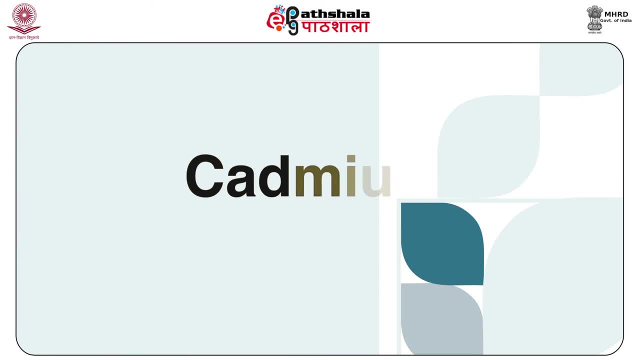 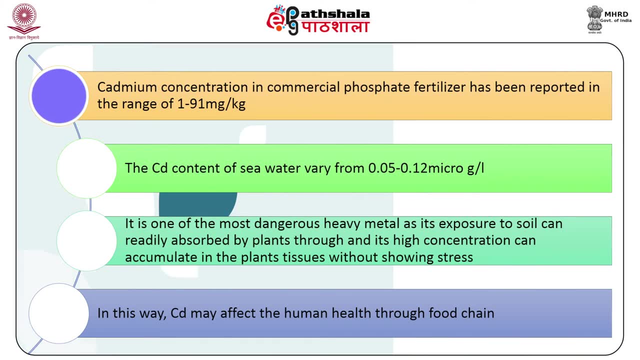 and brain functions and, ultimately, loss of blood and ultimately, death. Cadmium concentration in commercial phosphate fertilizer has been reported in the range of 1 to 91 mg per kg. The cadmium content of sea water vary from 0.05 to 0.12 microgram per litre. 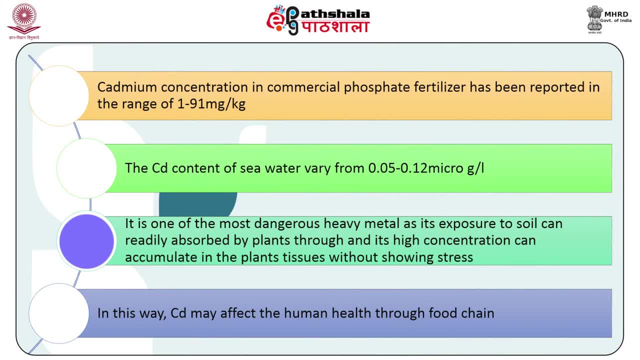 It is one of the most dangerous heavy metal as its exposure to the soil can radially absorb by plants through, and its high concentration can accumulate in the plant's tissue without showing stress. In this way, cadmium may affect the human health through food chain. 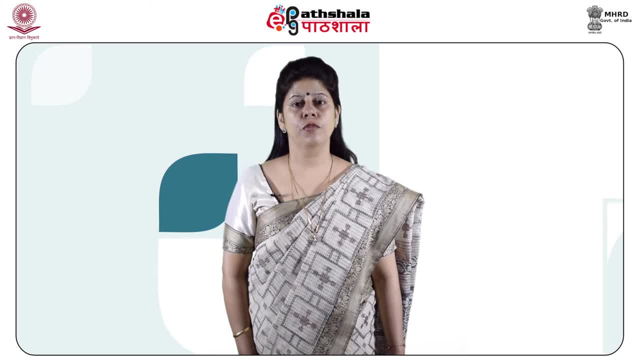 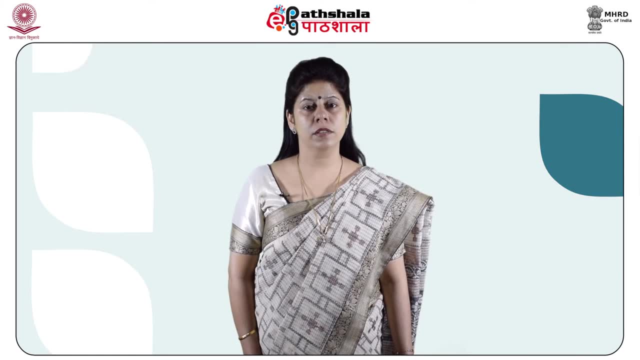 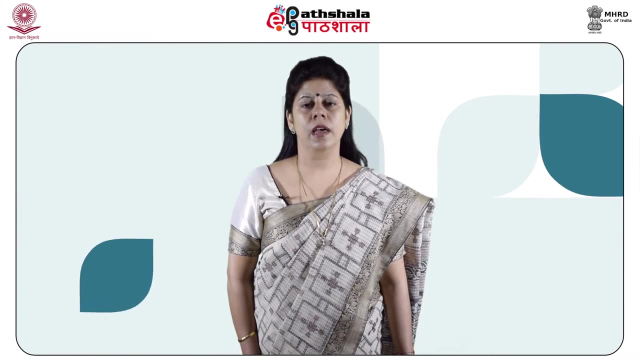 Sources of Cadmium. Cadmium enters the environment from mining and metallurgical operations, electroplating industries and other industrial activities Manufacturing vinyl, plastics, electrical contacts and many more Other. various anthropogenic activities are responsible for cadmium exposure to the soil. 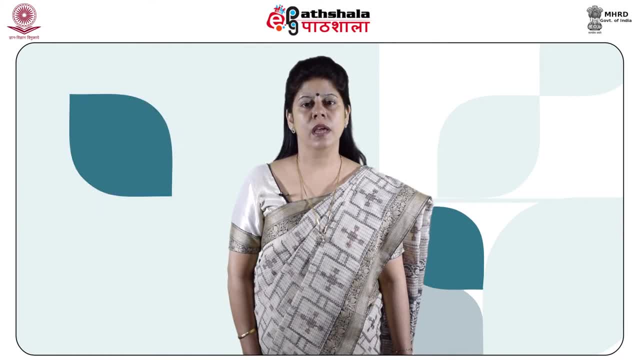 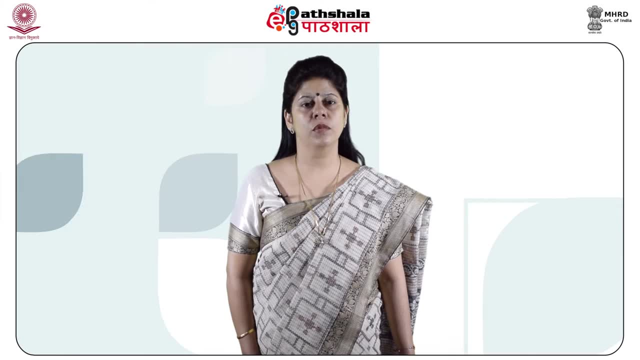 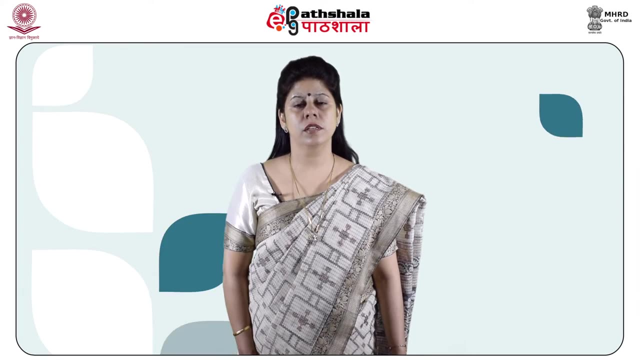 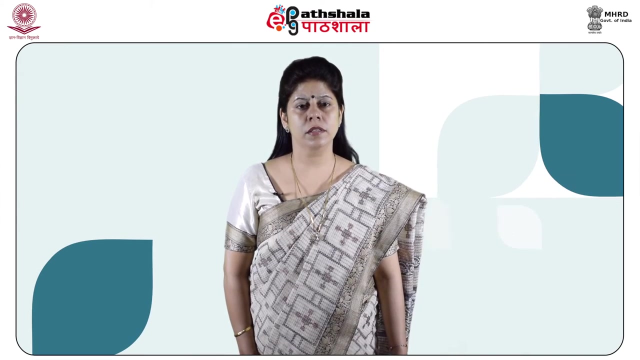 and may affect environmental health. Microorganisms maintain the fertility of the soil. The toxic effects of heavy metals like cadmium on soil and activities of microorganisms can be studied under controlled laboratory conditions. Soil from seaweed sludge containing number of higher metals and organic substances is. used to study the interaction between cadmium and microorganism. It may have a toxic effect on the microorganisms present in the soil which play an important role in maintaining the soil fertility. Health hazards caused by cadmium: 1. Cadmium toxicity may cause flu like symptoms such as chills, fevers and muscle aches. also, 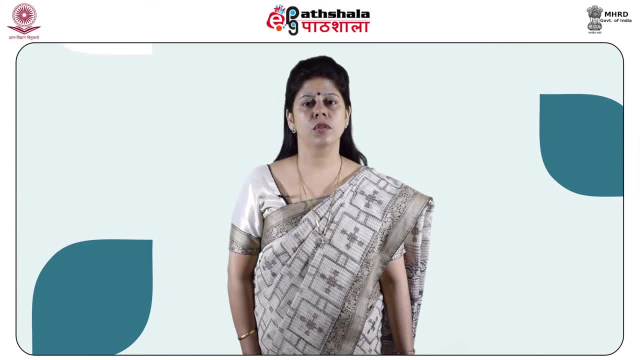 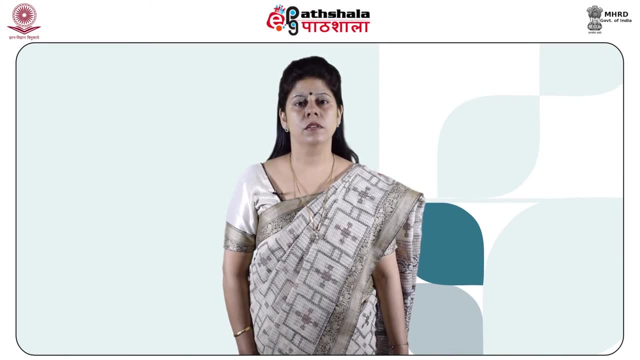 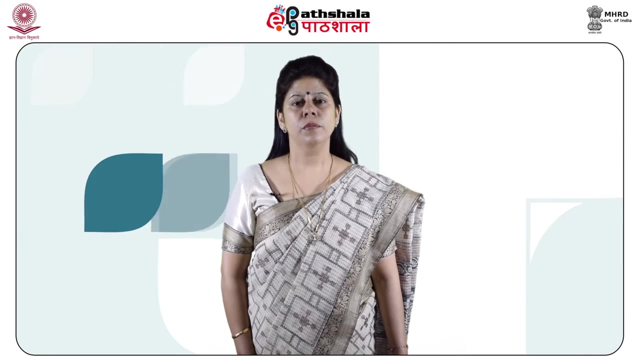 known as the cadmium blues. These symptoms may resolve after a week, but only if there is no danger to the respiratory system. Severe exposure results in tracheobronchitis, pneumonitis and pulmonary edema. Symptoms may be observed after some hours of exposure. 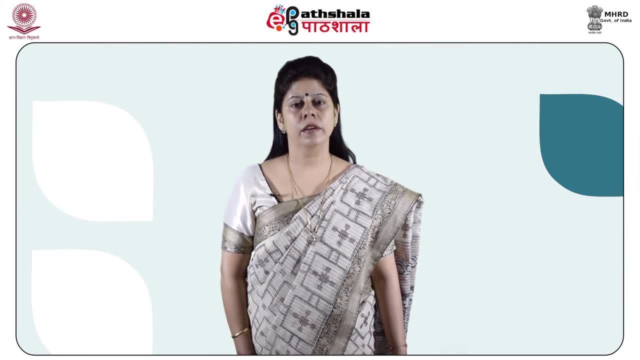 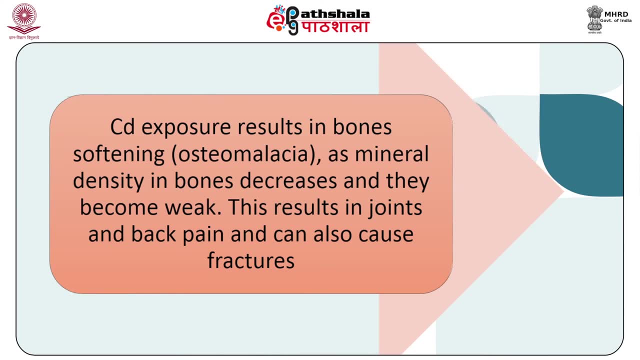 2. Cadmium exposure, which includes cough, headache, irritation in nose and throat, fever, chills and chest pains. 3. Cadmium exposure results in bone softening, causing osteomalacia, as mineral density in bones decreases and they become weak. 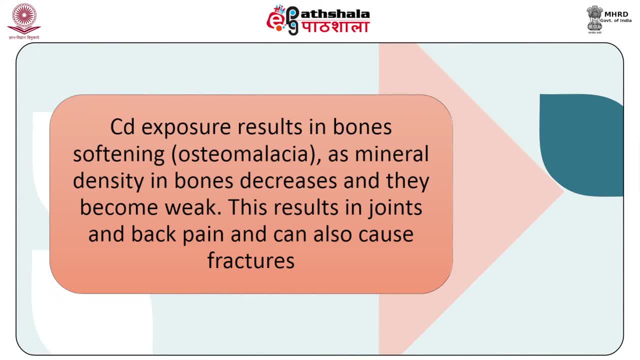 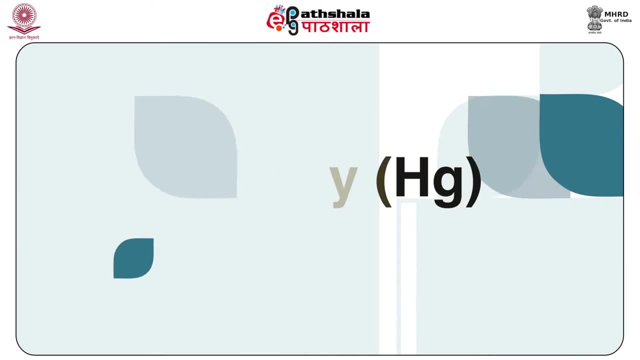 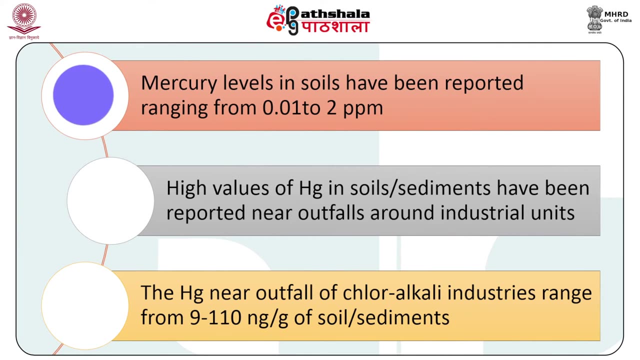 This results in joints and back pains and can also cause fractures. Now we will see The details of mercury contamination. Mercury levels in soils have been reported ranging from 0.01 to 2 ppm. High values of mercury in soils have been reported near outfalls around industrial units. 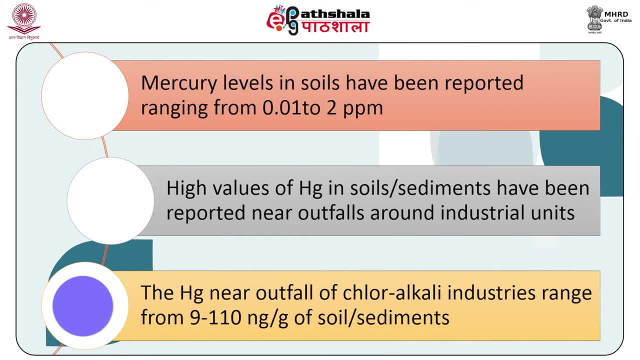 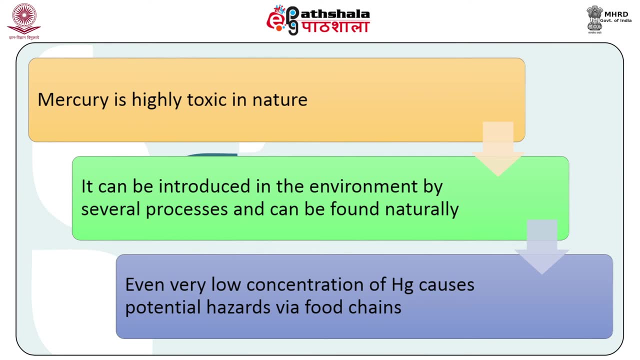 The mercury near outfalls of chloroalkali industries range from 9 to 110 mg per gram. This is the number of mercury in the soil. 4. Toxicity caused by mercury. Mercury is highly toxic in nature. It can be introduced in the environment by several processes and can be found naturally. 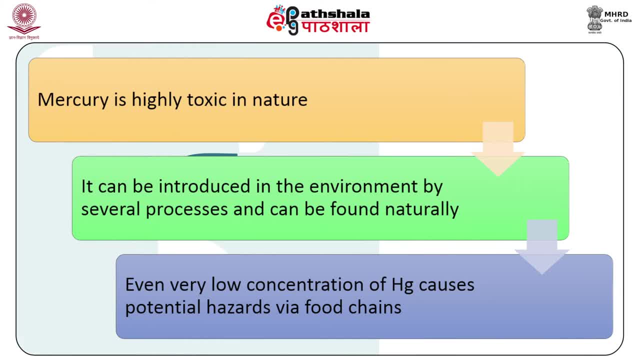 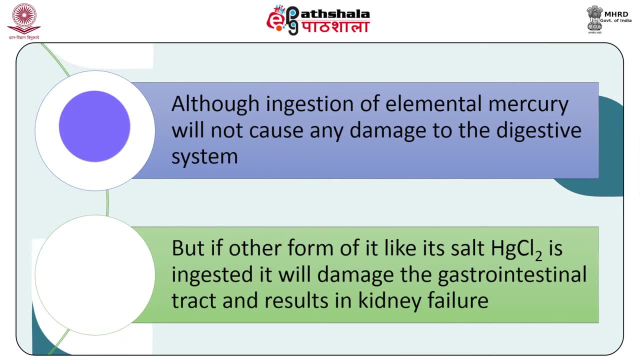 Even very low concentration of mercury causes potential hazards via food chains, Although ingestion of elemental mercury will not cause any damage to the digestive system. But in the case of mercury in the body, the food chain may also be affected. But if other form of it, like its salt HgCl2, is ingested, it will damage the gastrointestinal. 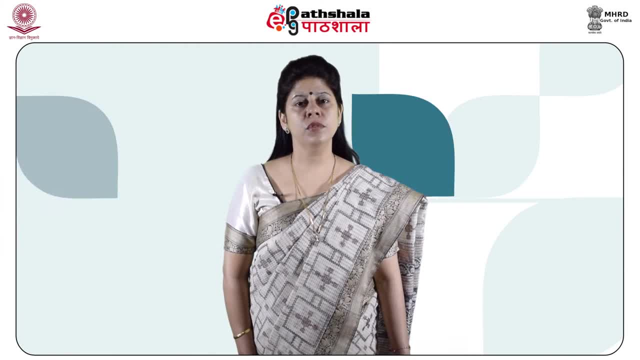 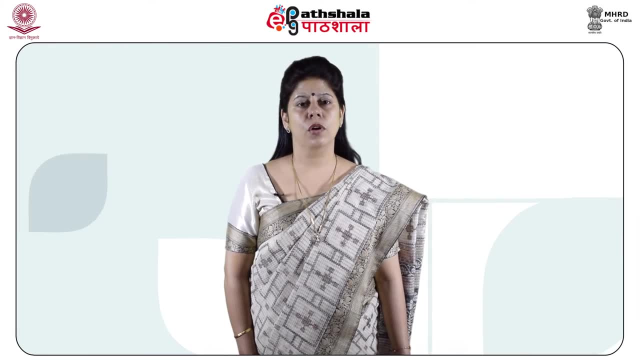 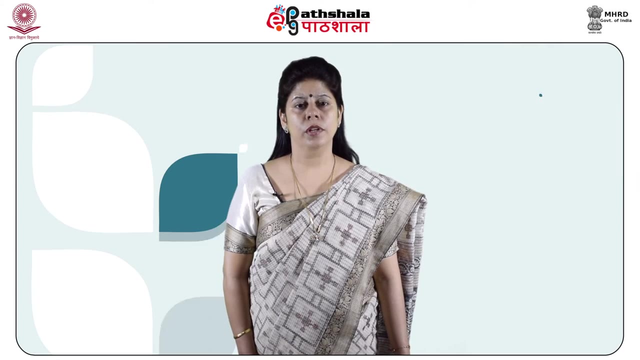 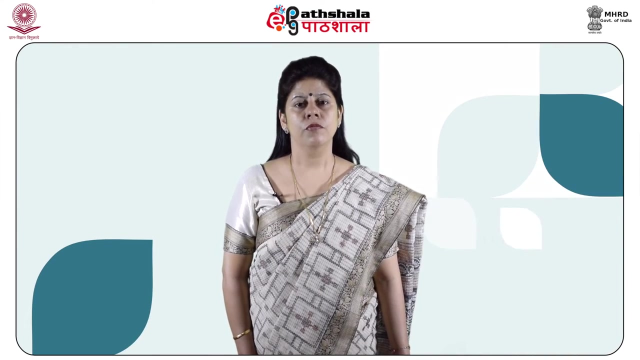 tract and results in kidney failure. Maximum source of mercury is in chloralkali industry, mercury catalyst in the manufacture of vinyl chloride, plastic and acetaldehyde, Chemical industries for the production of battery lamps and circuit breaker, pulp and paper industries, paints, fungicides, jewellery, pharmaceuticals and in research processes. 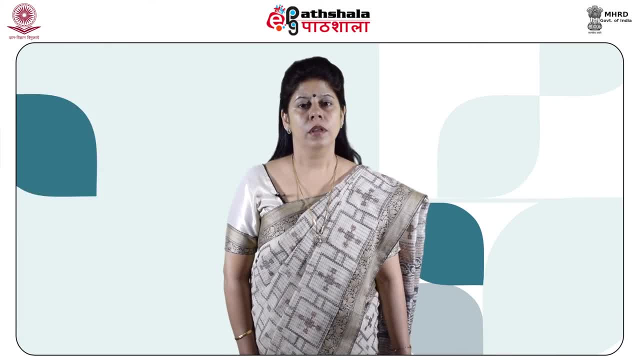 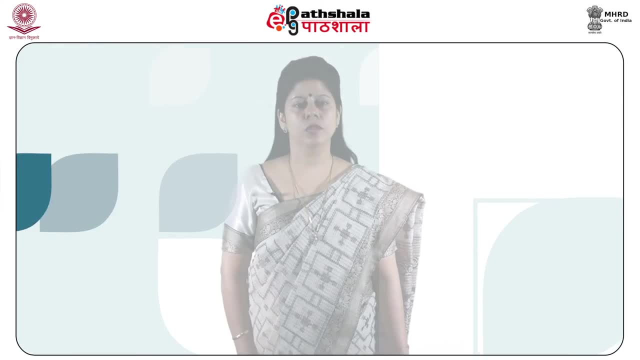 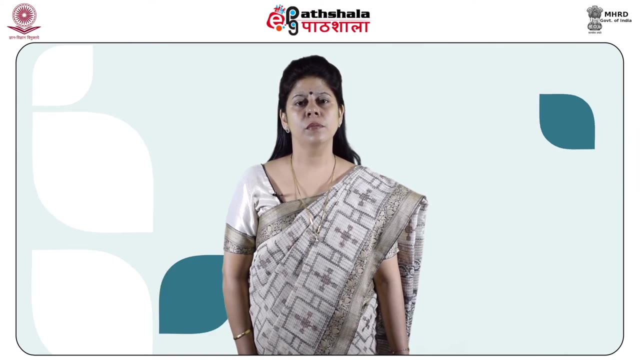 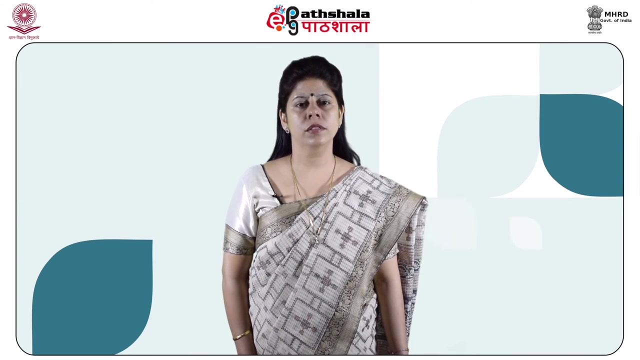 Thermometer contain elemental mercury. therefore, if broken down, released mercury in zero state. Health hazards caused by mercury: Continuous inhalation of its vapours results in tremors, Gingivitis. Elemental mercury is comparatively less toxic than methylmercury that is found in high concentration. 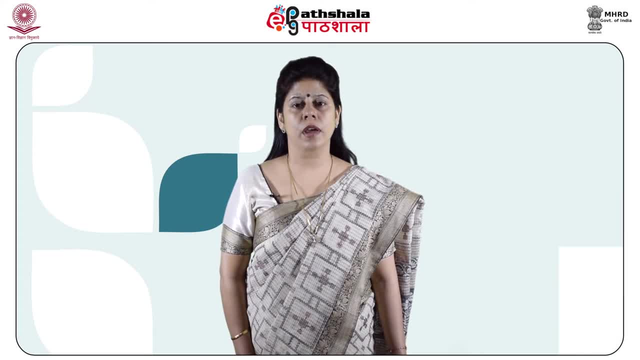 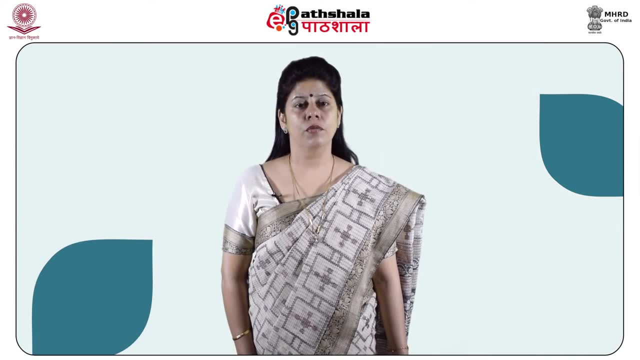 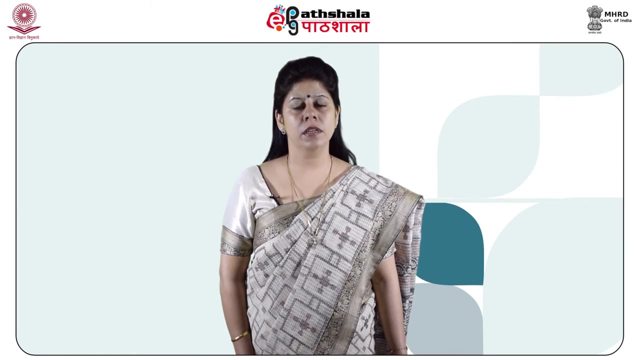 near gold mine sites as it is used to extract gold. If fish contaminated with methylmercury is eaten by people and wildlife, it will affect the immune system. It also damages the genetic, enzymatic and nervous system of the body. Thank you, 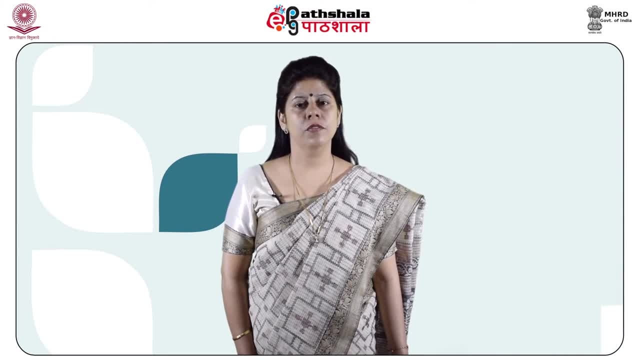 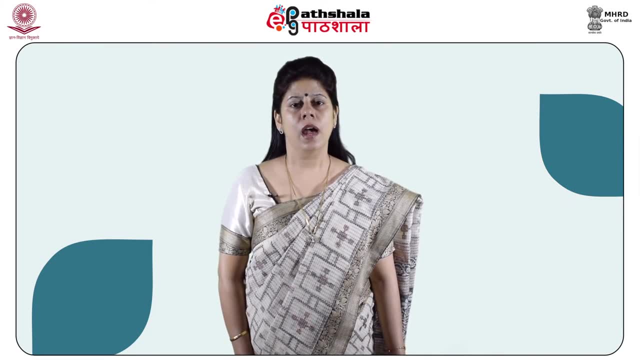 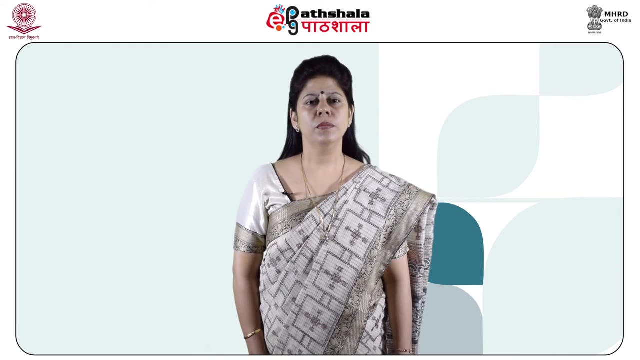 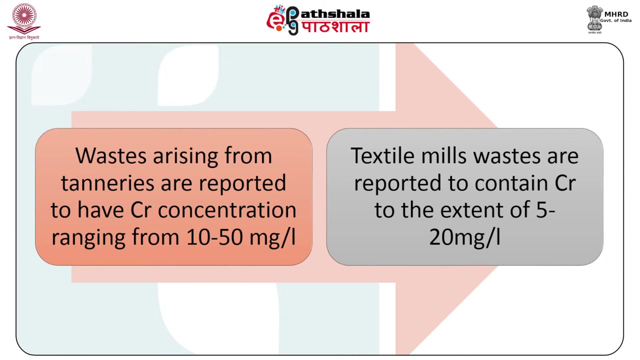 Developing embryo being very sensitive, mostly get affected by it. It is more dangerous because it is ingested readily and excreted slowly than any other form of mercury. Chromium- Optimum concentration of chromium. Waste arising from tanneries are reported to have chromium concentration ranging from 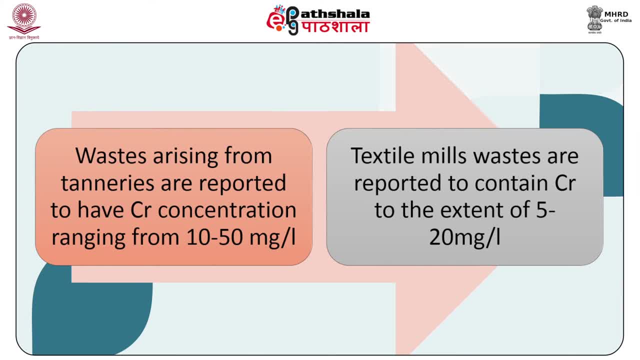 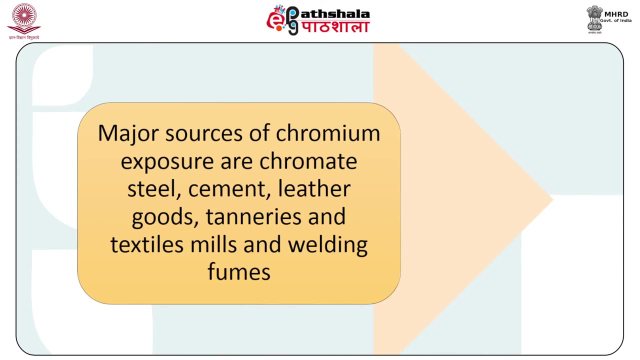 10 to 50 mg per litre. Textile mills waste are reported to contain chromium to the extent of 5 to 20 mg per litre. Major sources of chromium exposure are chromate steel, cement, leather goods, tanneries and textile mills and welding fumes. 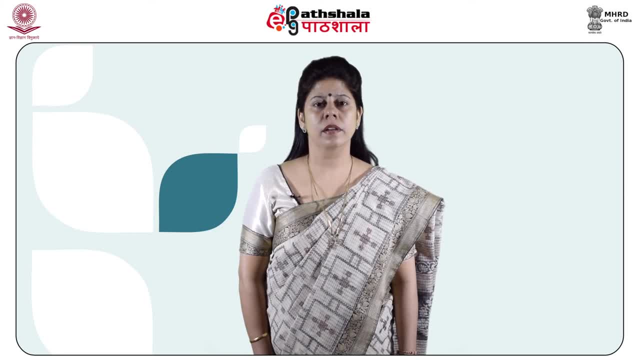 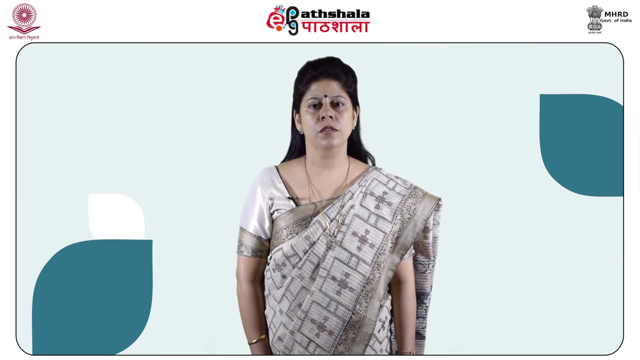 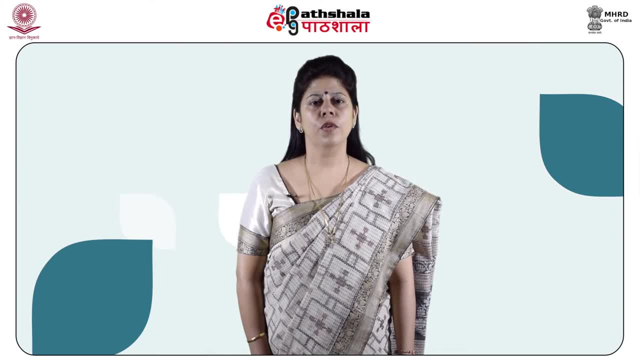 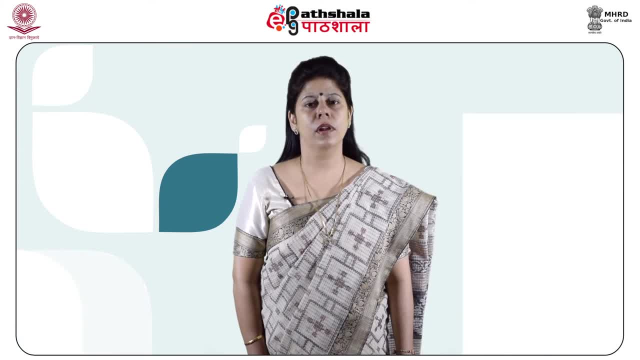 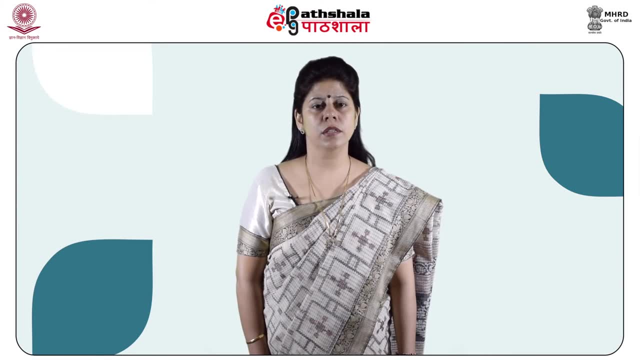 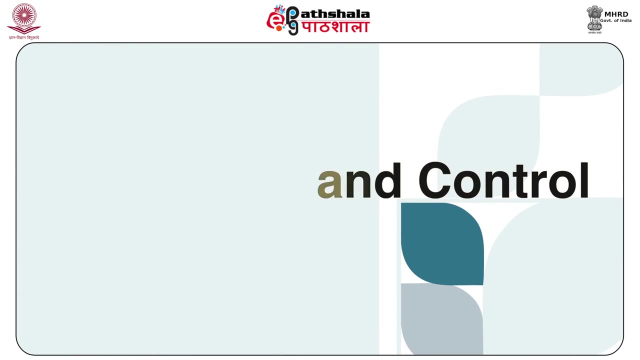 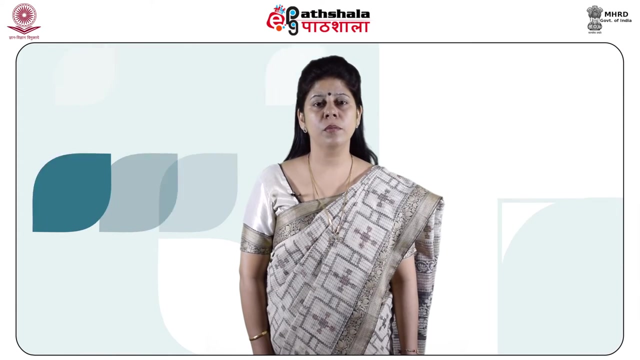 Exposure to the chromким dust increases the chances of lung cancer, and oral administration of 50 ppm of chromate has been associated with growth, depression, liver and kidney damage. Now we will see what are the preventions and control. The pollution caused by heavy metal is a critical because it is extremely expensive and difficult. 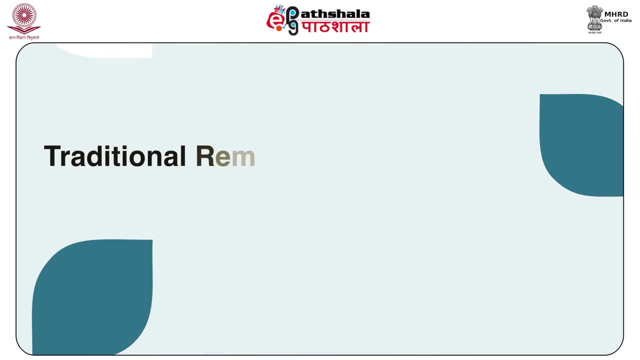 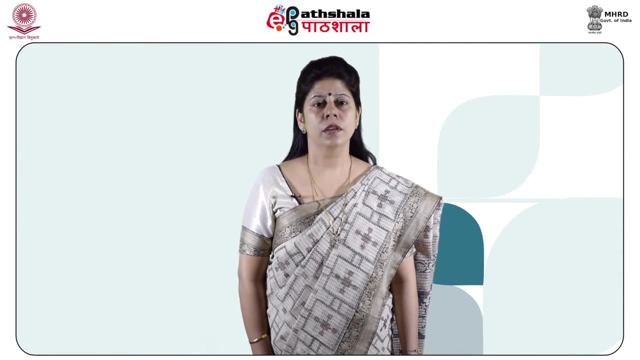 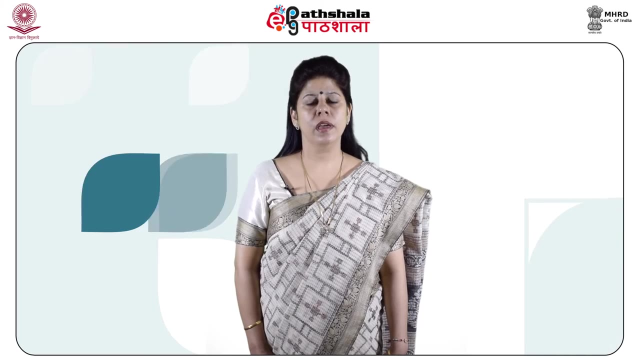 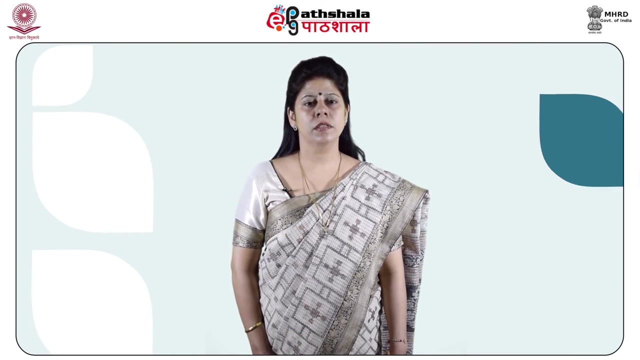 to clean the soil contaminated by it. Traditional remediation of contaminated soil. The metals that contaminate the environment cannot be easily removed as they do not degrade like organic molecule, But microorganism can be used to transform mercury and selenium. Traditional treatments are expensive when the concentration of contaminated soil is. 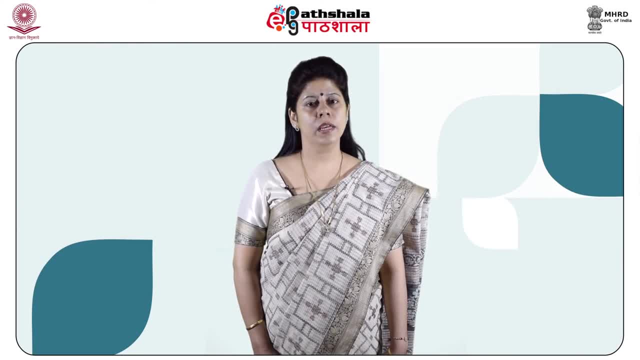 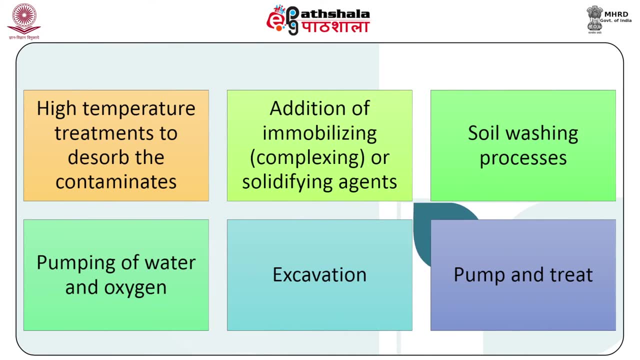 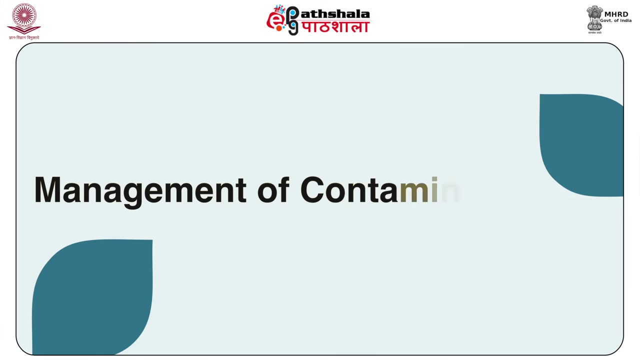 large Treatment can be done in-situ or ex-situ, such as high-temperature treatment to deabsorb the contaminants, addition of immobilizing or solidifying agents, soil washing processes, pumping of water, Water and oxygen excavation pump and treat. 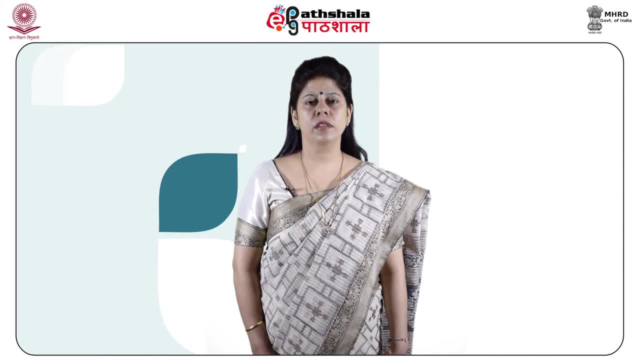 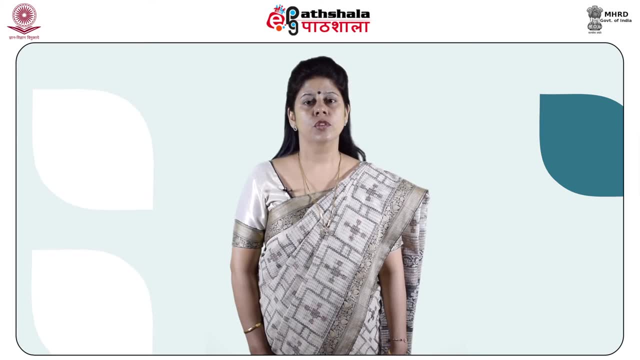 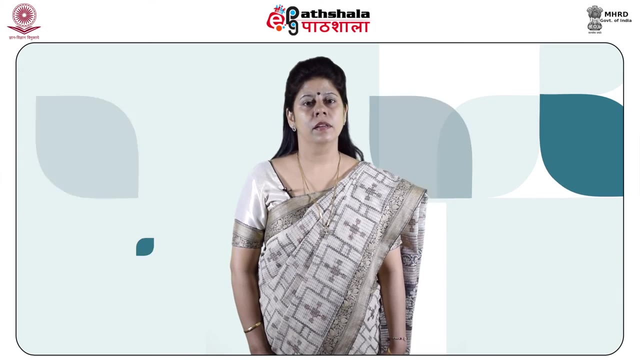 Management of contaminated soil. It is an effective method to prevent uptake of pollutants by plants by leaving them in soil. In this case, soil act as a sink, which results in breaking of soil, plant, animal or human cycle and exerts toxic effects. Management practices are not helpful in removal of contaminated soil. Treatment can be done in-situ or ex-situ, such as high-temperature treatment to deabsorb the contaminants, addition of immobilizing or solidifying agents, soil washing processes, pump and treat. 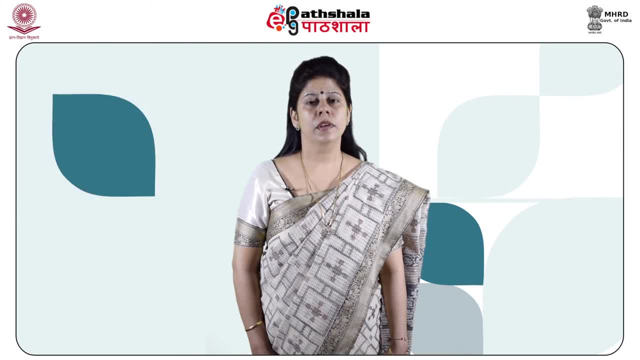 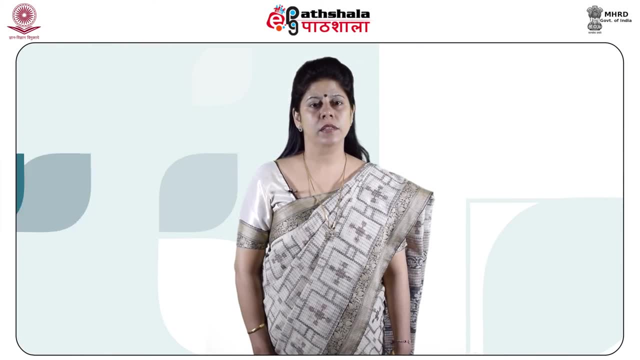 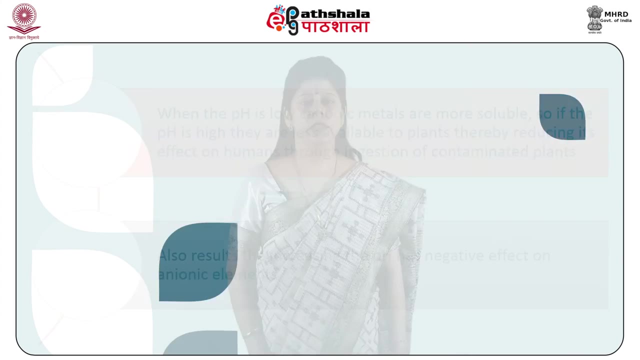 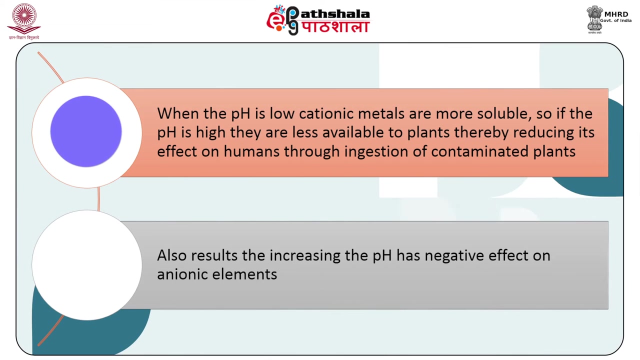 Management of contaminated soil. It is not helpful in removal of heavy metal contaminants, but will help in reducing the potential for adverse effects from the metals, depending upon the kind of metal. Create planting blocks因為土地. Felipe M sauce effect on humans through ingestion of contaminated plants. 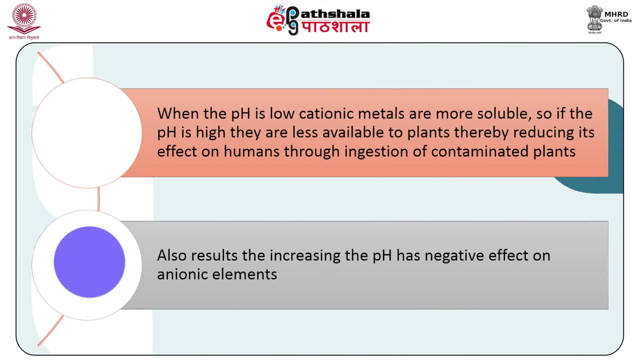 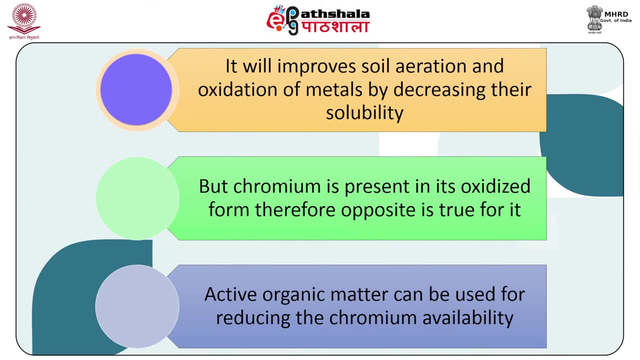 Also results. the increasing the pH has negative effect on anionic element Draining wet soils. It will improve soil aeration and oxidation of metals by decreasing their solubility. But chromium is present in its oxidized form. therefore opposite is true for it. 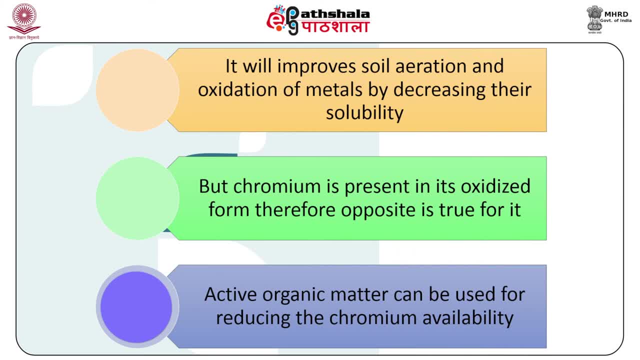 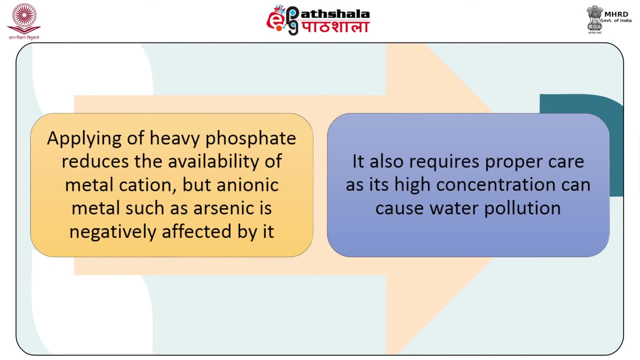 Excessive organic matter can be used for reducing the chromium availability Applying phosphate. Applying of heavy phosphate reduces the availability of metal cation, but anionic metal such as arsenic is negatively effected by it. It also requires proper care, as its high concentration can cause water pollution. 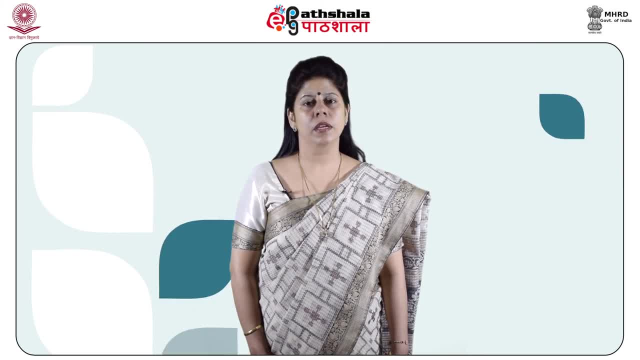 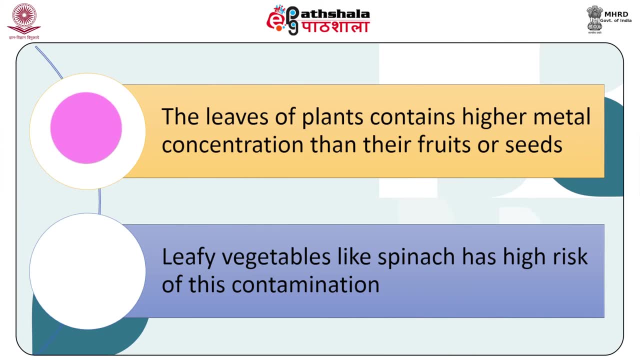 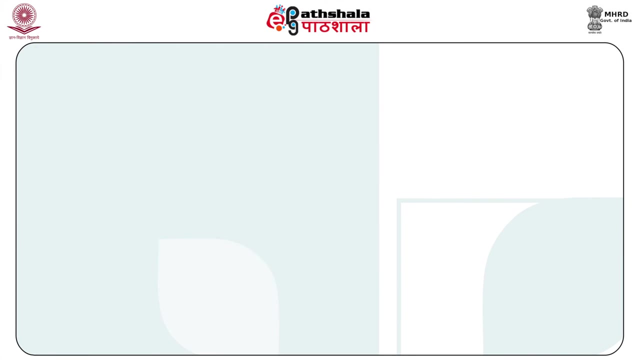 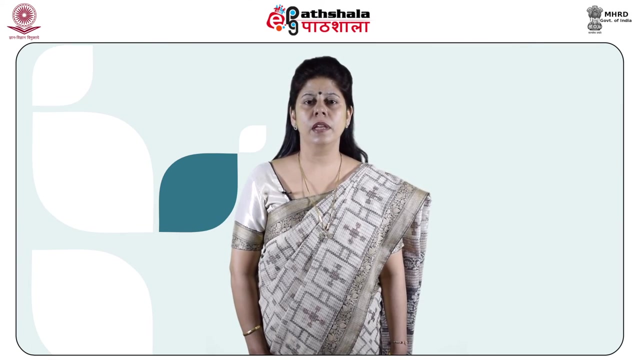 Selection of plants for use On metal contaminated soil. The leaves of plants contains higher metal concentration than their fruits or seeds. Leafy vegetables like spinach have high risk of this contamination. Plants for environmental cleanup: It is observed that plants can help in cleaning up of contaminated soil. 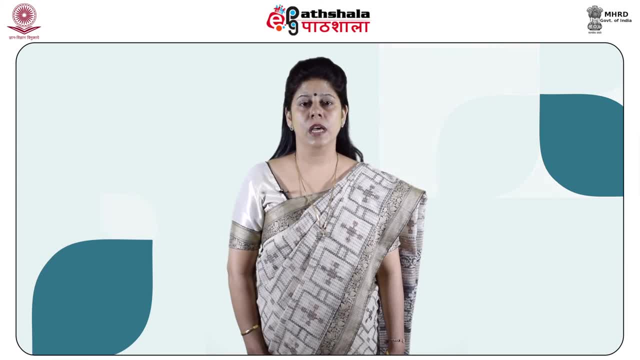 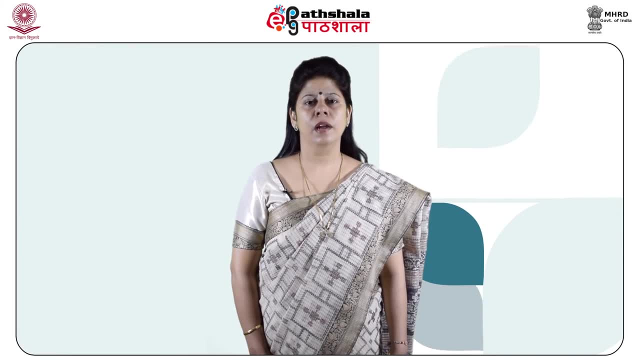 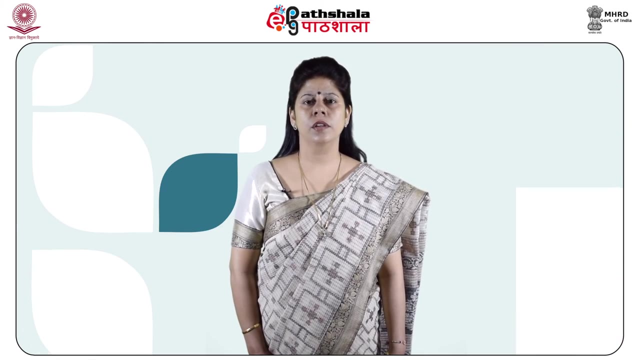 This process of removing soil pollutants, For example, Pesticides, heavy metals, solvents, polyaromatic hydrocarbons, crude oils and landfill leachates by plants, is known as phytoremediation. In the recent study in Kuwait, it is seen that wild flowers helps in degradation of hydrocarbons. 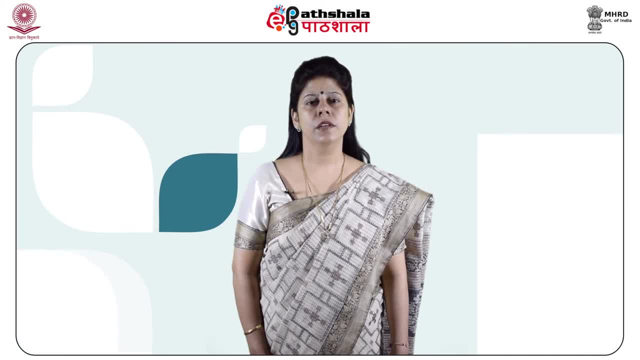 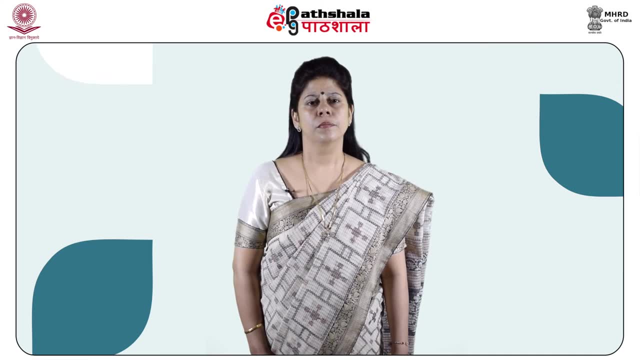 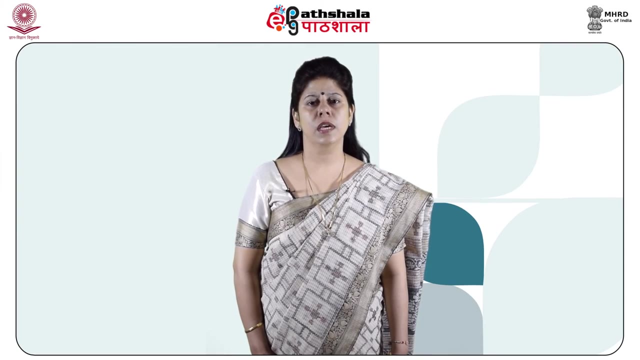 from an oil spill. Pesticides emanation compounds such as TNT can be removed by hybrid poplars. Pesticides emanation compounds such as TNT can be removed by hybrid poplars Plants for treating metal contaminated soil Plants can be used for removal of metal contaminants from soil and water. 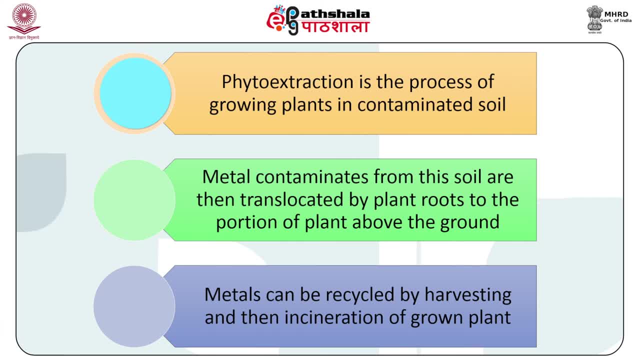 Phyto extraction is a process of growing plants in contaminated soil. Metal contaminants from this soils are then translocated by plant roots to the portion of plants above the ground. Metals can be recycled by harvesting and then incineration or by composting. 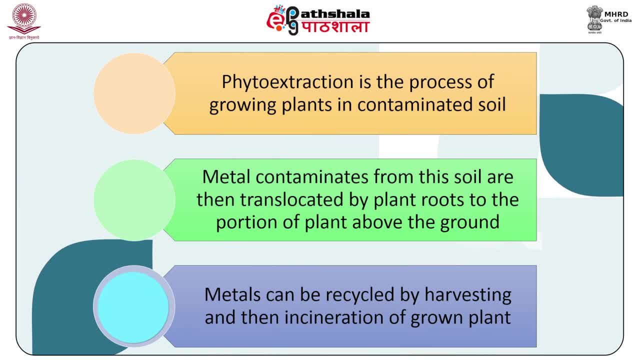 Plants for the use of phyto extract. Plants can be used for the use of phyto extract. If you are not familiar with phyto extract, phyto extract is a chemical that is used in soil treatment. It is said that it is used in the chemical production of soil. 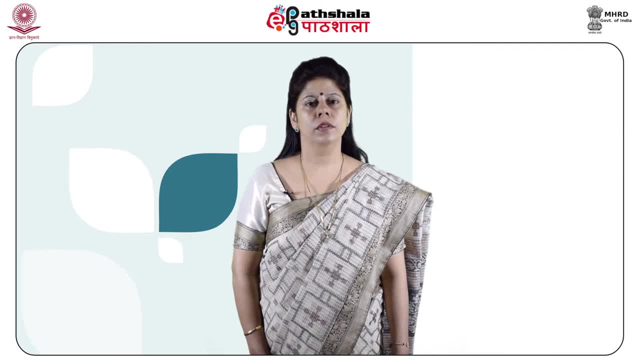 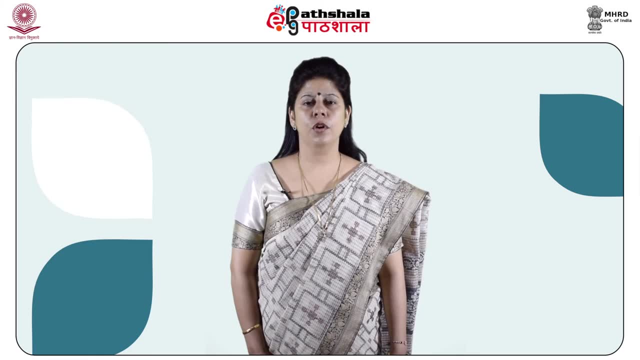 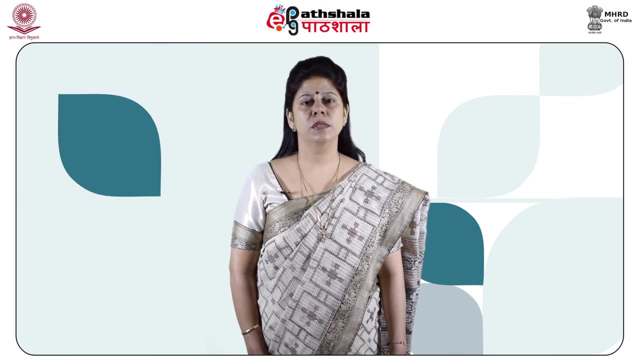 of grown plants- There are many crops growth cycles, which decreases the contamination level of the soil. Ash obtained from plants incineration must be disposed of in a landfill, but its volume is much smaller than the volume of contaminated soil if dug out and removed for. 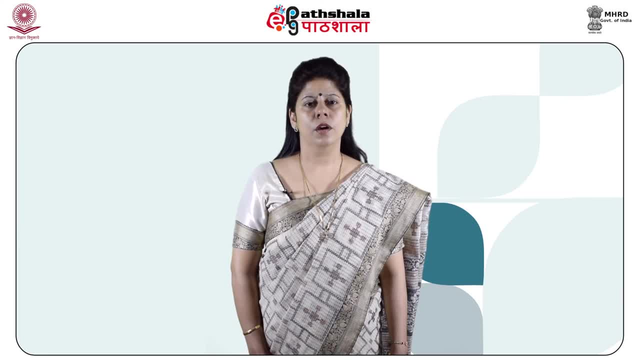 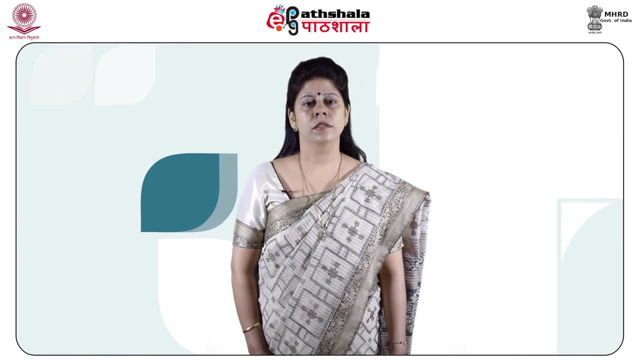 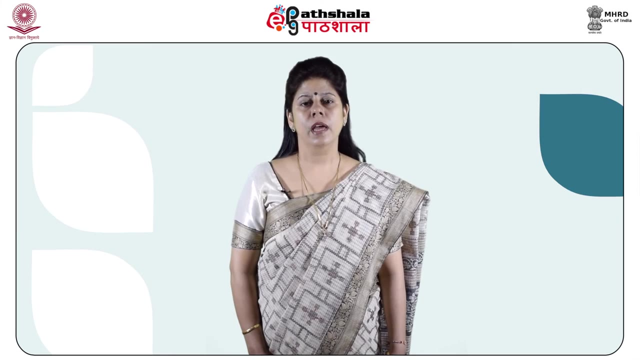 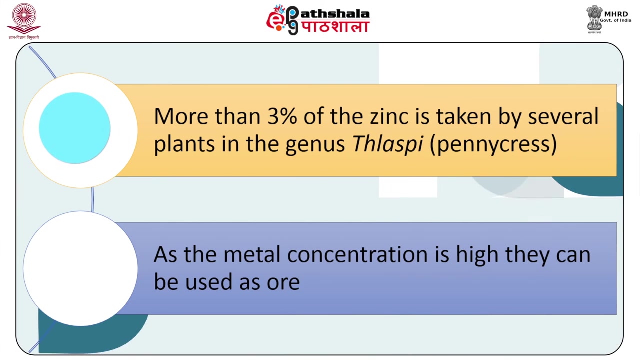 treatment. Hyperaccumulators are plants which absorbs metal in higher concentration. therefore can be used as phyto-extractors. Metal such as nickel, zinc and copper can be easily phyto-extracted. More than 3% of the zinc is taken by several plants in the genus Thulspea Penigris Thulsa. 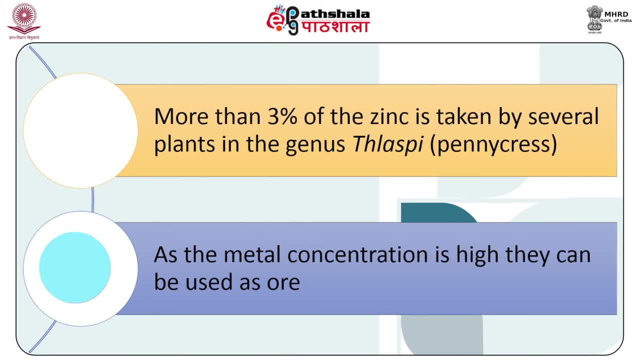 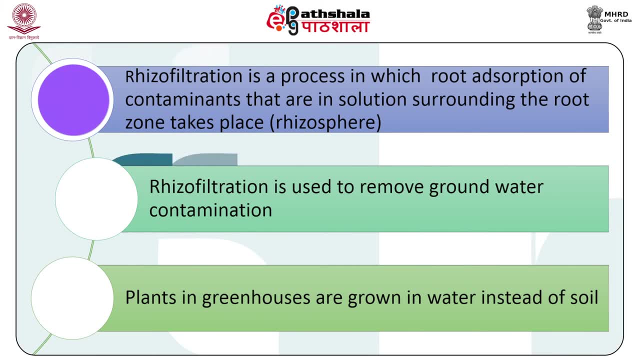 Thulsa, As the metal concentration is high, they can be used as ore Resofiltration. Resofiltration is a process in which root adsorption of contaminants that are in solution surrounding the root zone takes place- Resofiltration. 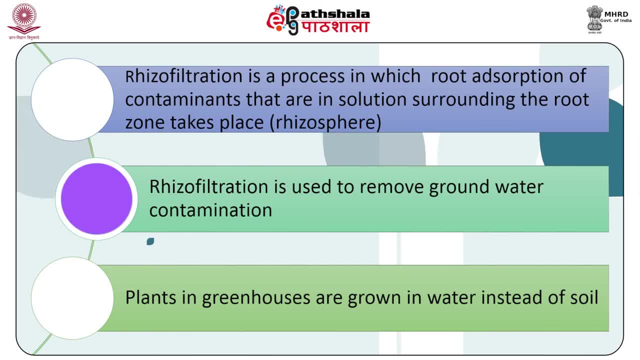 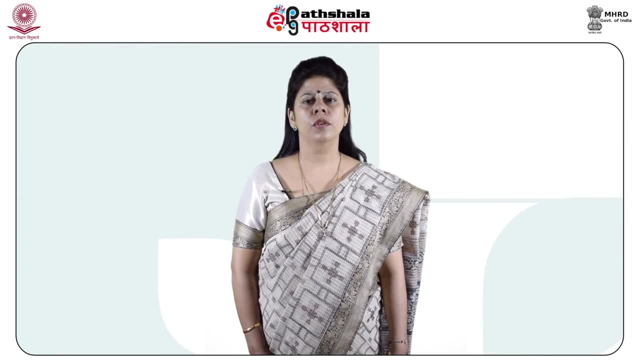 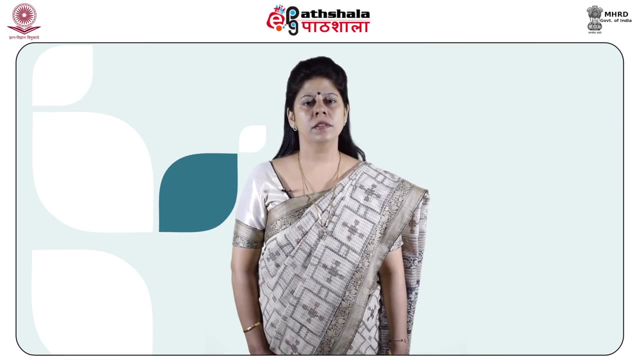 is used to remove ground water contamination. Plants in greenhouses are grown in water instead of soil For this. plants are grown on contaminated ground water and roots takes up this contaminated water. The plants are harvested along with roots if it gets saturated with the contaminant. 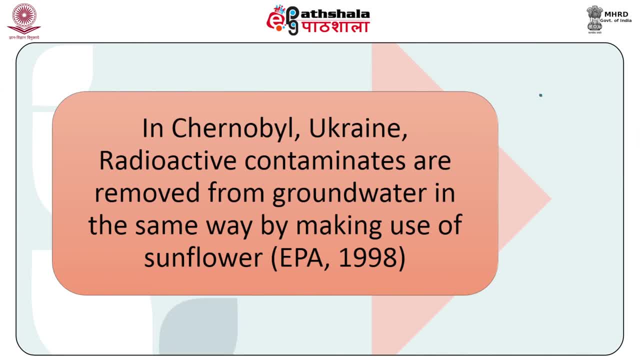 In Chernobyl, Ukraine. radioactive contaminants are removed from the ground water in the same way by making use of sunflower Phytostabilization. Phytostabilization is used for animal- christening. Phytostabilization is an environment where plants can be easily metabolized with Madisonian. 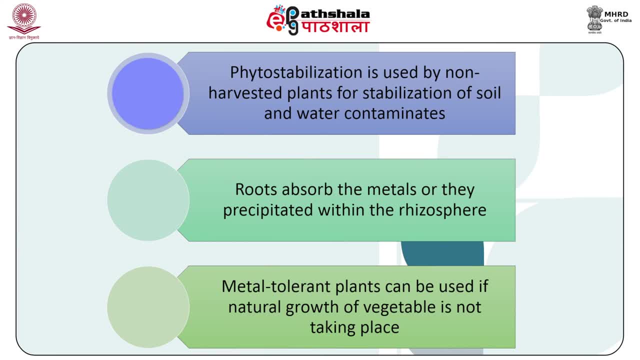 used by non-harvested plants for stabilization of soil and water contaminants. Roots absorb the metal or they precipitated within the rhizosphere. Metal tolerant plants can be used if natural growth of vegetable is not taking place. This will decrease the risk. 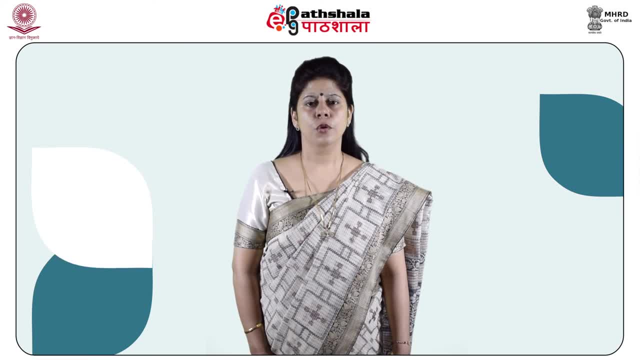 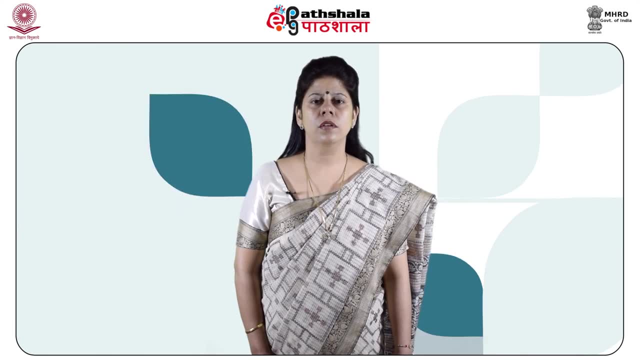 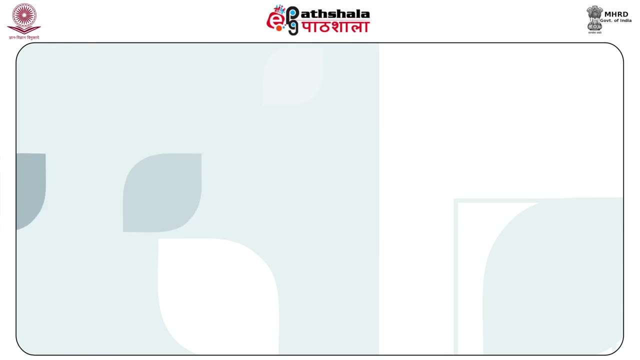 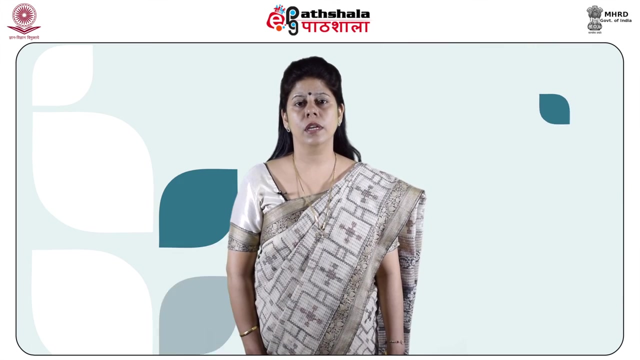 of soil erosion. Phytostabilization basically reduces the velocity by which contaminants are growing into the ground, water or the air. Example of disposal: Plants for treating metal contaminated soil. Lead is considered to be the most toxic metal for soil. Naturally, the lead is not absorbed by plants. It requires. 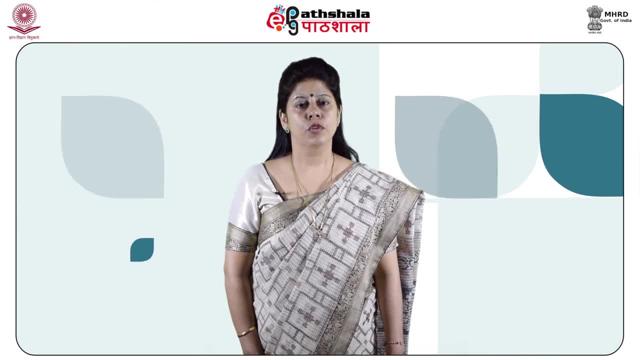 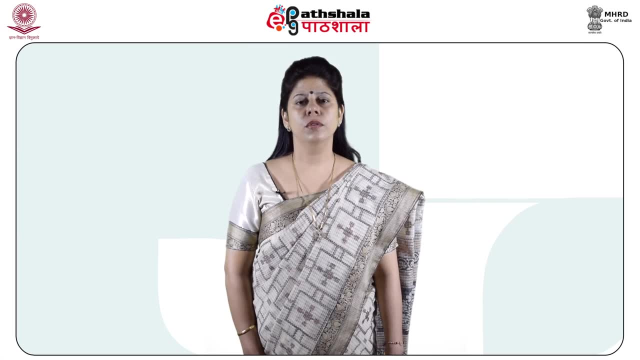 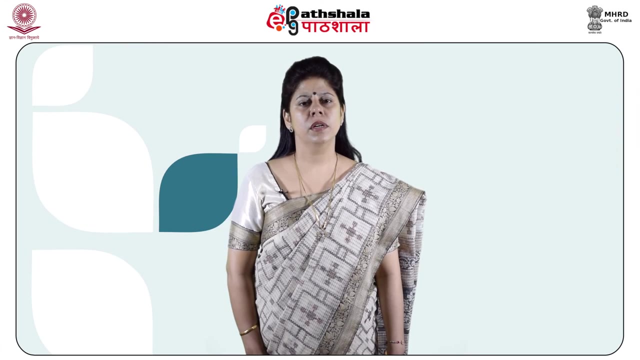 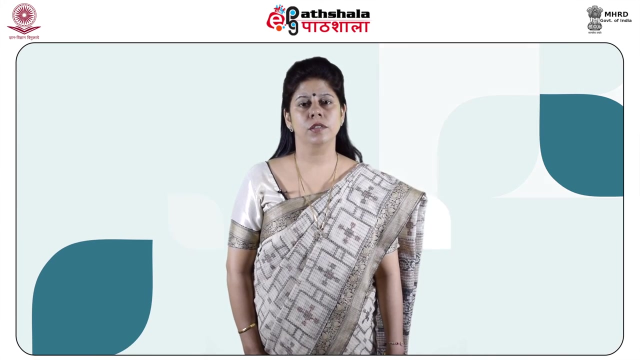 a chelator such as ADTL, Which makes the adsorption of lead by the plants possible. Lead can be extracted by using Indian mustard. Phytotec has reported that in New Jersey, Indian mustard is used in order to reduce the lead contamination sites below the industrial standards Plants. 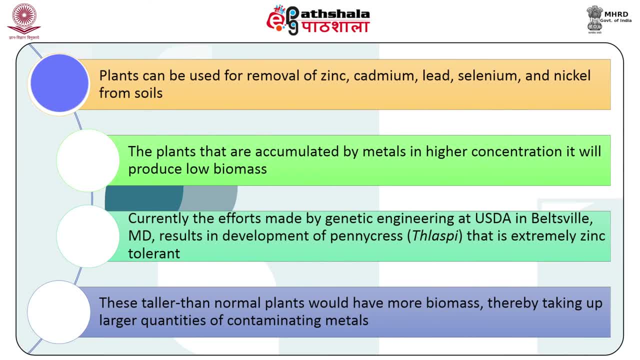 can be used for removal of zinc, cadmium, lead, selenium and nickel. The plants that are accumulated by metal in higher concentration will produce low biomass. Currently, the efforts made by genetic engineering at USDA in Beltsville results in development of a pennycress known as thulspe that is extremely zinc tolerant. These taller than normal plants- 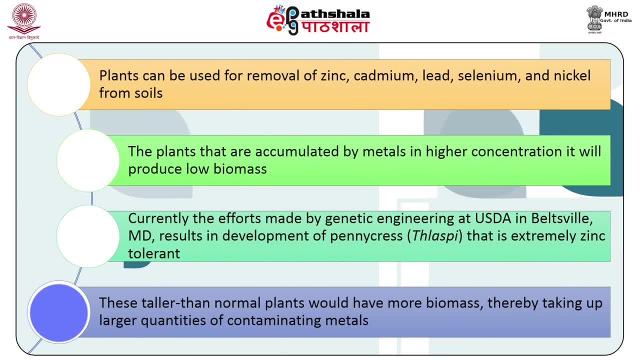 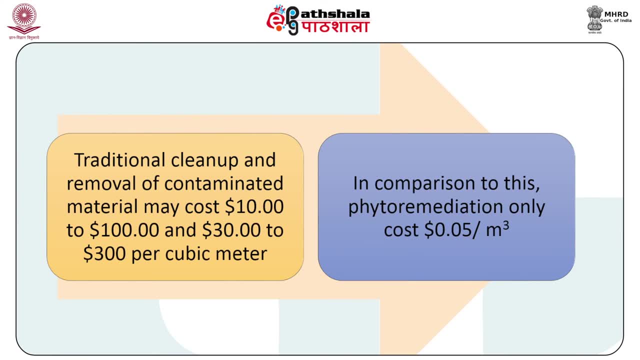 would have more biomass. In addition, thulspe can be used to clean the soil by taking up larger quantities of contaminating metals. Traditional cleanup and removal of contaminated material may cost $10 to $100 and $30 to $300 per cubic meter. In comparison to this phytoremediation cost, 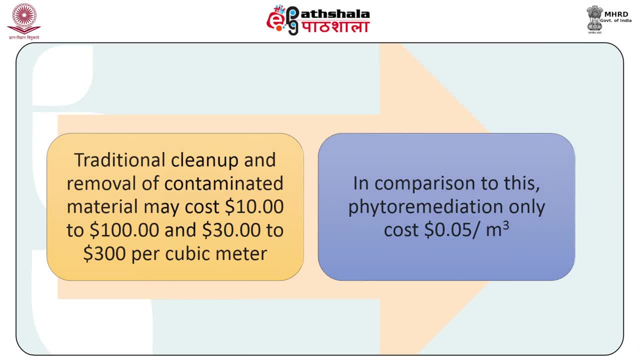 only $0.05 per meter cube. Summary: 1. Soil is an essential material. 2. Soil is an essential material. 3. Soil is an essential material. 4. Soil is an essential material. 5. Soil is an essential material. 6. Soil is an essential material. 7. Soil is an essential. 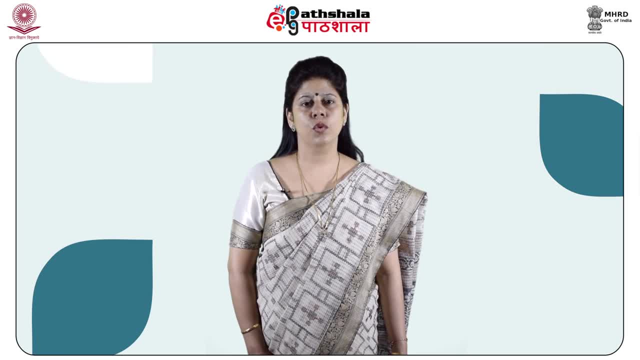 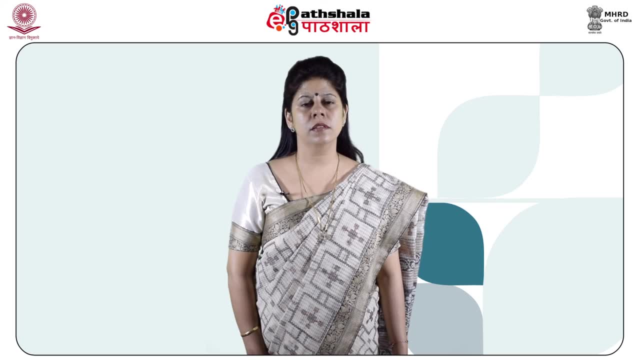 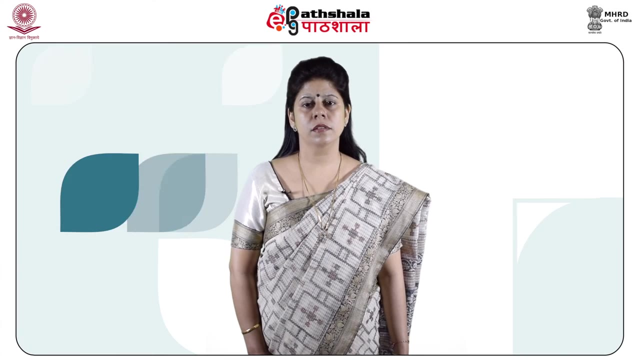 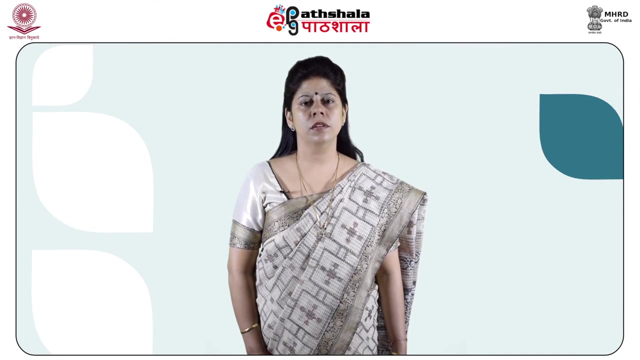 component of our environment, and its quality can be maintained by land management. Metals are the natural substances that are found in soil at low levels. Nevertheless, the metals emitted by the processes such as mining, manufacturing and the use of synthetic products result in contamination in urban and agricultural soil. They remain in the 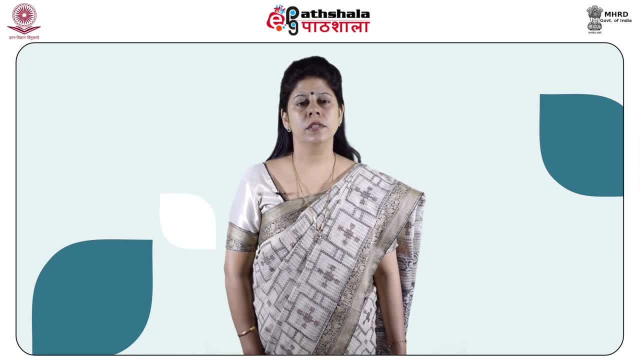 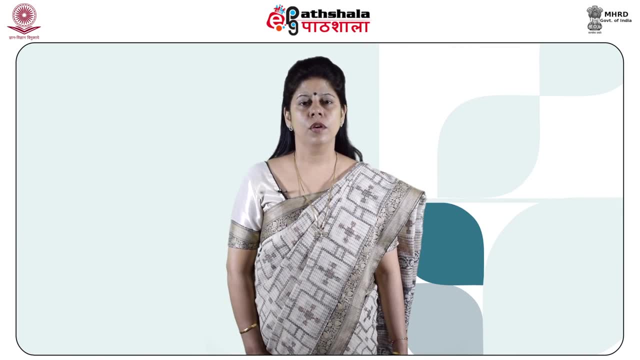 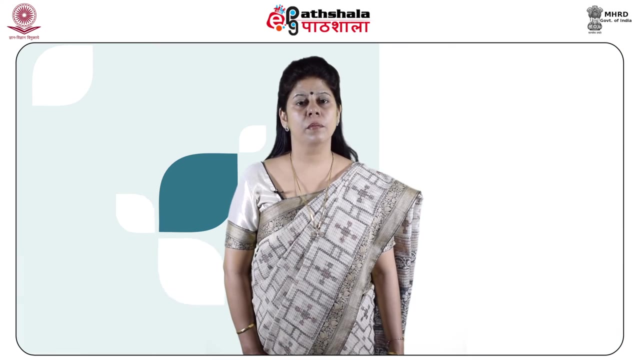 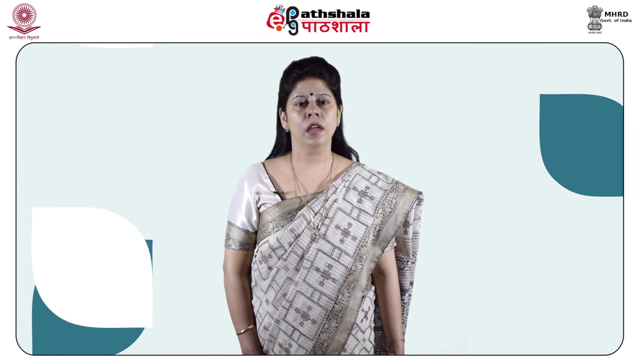 soil indefinitely, as the metals do not degrade. The problem-causing metallic elements exist in soil, such as positively or negatively charged species. Mercury, cadmium, lead, nickel, copper, zinc, chromium and manganese are the cations in soil. On the other hand, arsenic, molybdenum, selenium and boron are the anionic compounds. present in the form of arsenic, cadmium, nickel, copper, zinc, chromium and manganese. On the other hand, arsenic, molybdenum, selenium and boron are the anionic compounds present in the form of arsenic, cadmium, lead, nickel, copper, zinc, chromium and boron. 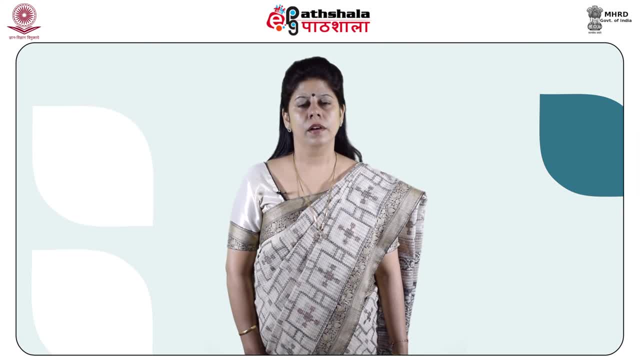 On the other hand, arsenic, molybdenum, selenium and boron are the anionic compounds present in the form of arsenic, cadmium, lead, nickel, copper, zinc and boron, Natural and anthropogenic. both the sources are responsible for environmental pollution. 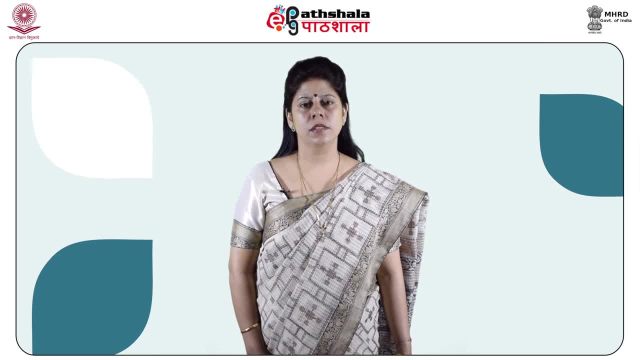 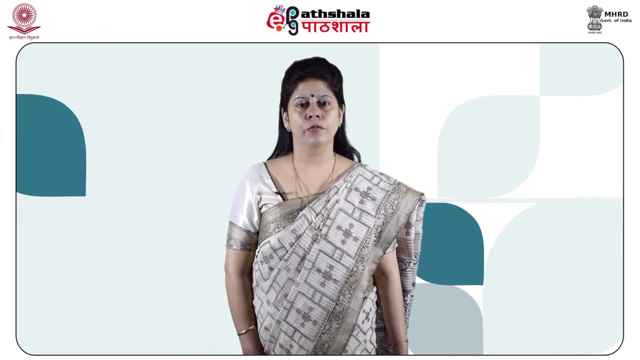 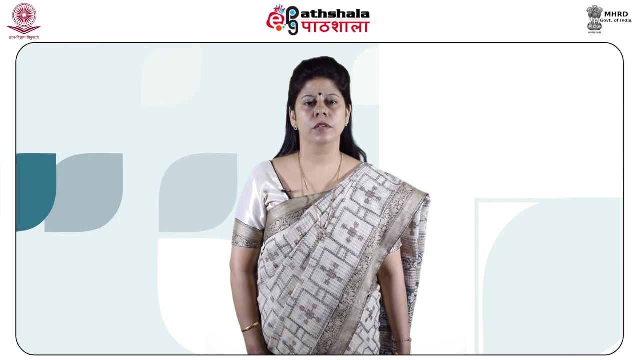 which are hazardous to environment. Metal toxicity is a deadly effect of certain metals, in definite forms and doses, on life form. Some of the metals are very toxic as they form soluble compounds poisonous in nature. Generally, the laxative compounds in the form of arsenic, ferritin or ferritin break down the natural elements of the soil into a rich